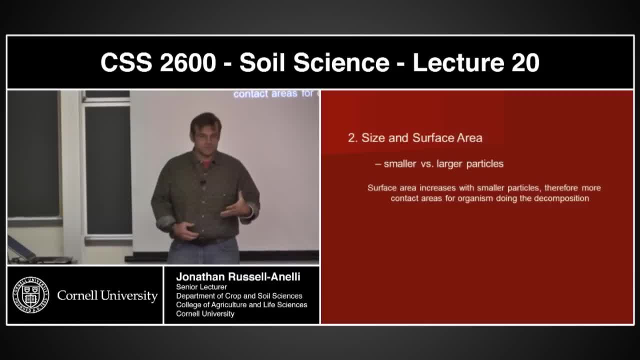 think about it. okay, If we look at the particles, the size of the material that's being decomposed, larger particles have less surface area per volume. Does that make sense? Kind of like when we start cutting up the soil: the finer the 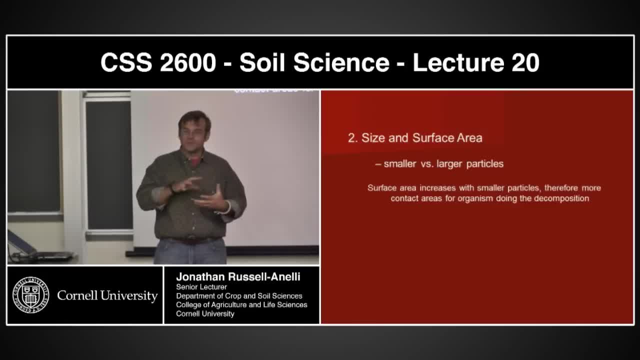 texture, the more surface area has to be. That's what we have for the volume, okay? Well, if that's the case, the smaller- sorry, the smaller- the particle is, the more surface area there is for the organisms that are going to be doing the decomposition to actually access that. 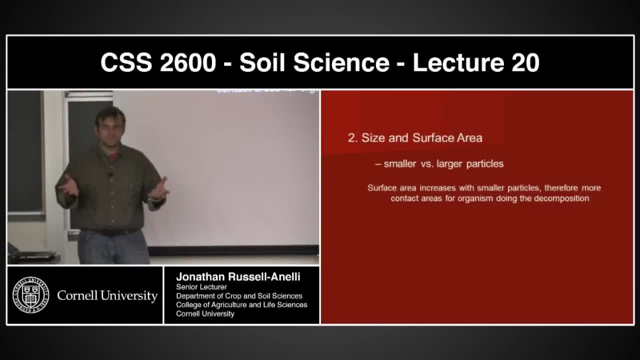 particle Makes sense. okay, So in reality, the reality is that surface area does in fact control decomposition rates. Smaller things decompose faster than larger things. in general, okay, Now you have to take into account placement, CN ratio and the nature of the recalcitrance of the 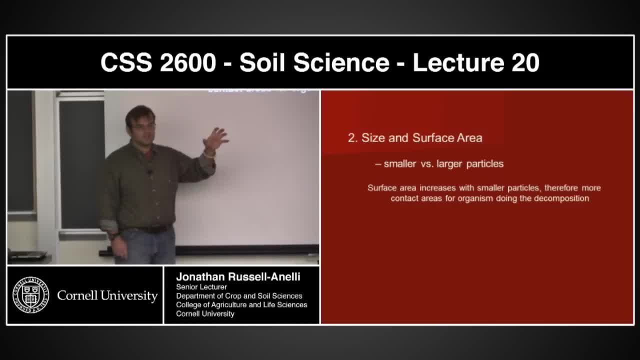 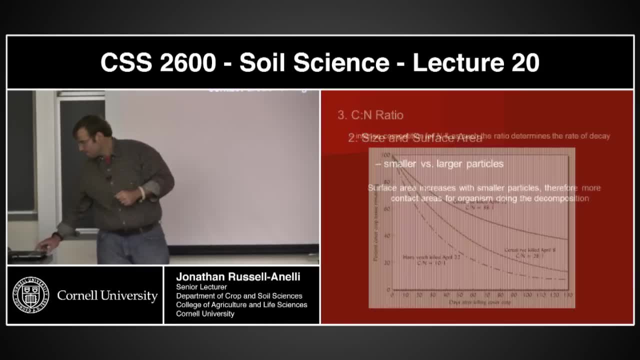 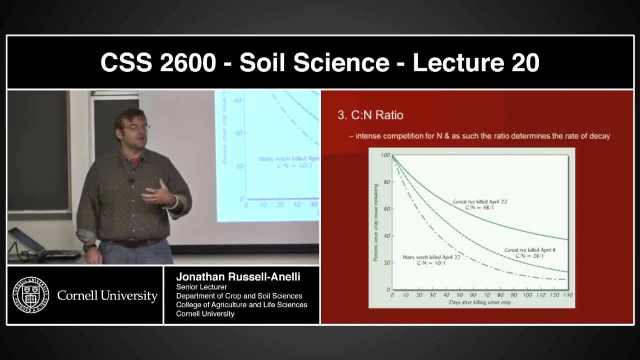 material as well, but if you just look at size, smaller is faster than bigger when it comes to decomposition. okay, All right. the next thing is: this is sort of the third controlling factor, and this is carbon-nitrogen ratios, CN ratios- okay, 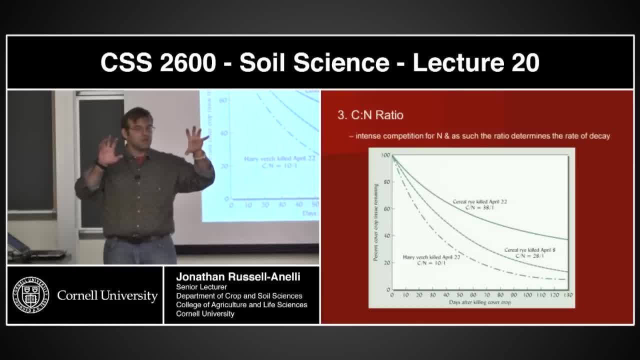 A CN ratio is basically how much carbon there is relative to nitrogen. The larger the number, the more carbon there is to nitrogen- okay. The smaller the number, the less carbon there is to nitrogen- okay, There's intense. you gotta sort of think about. 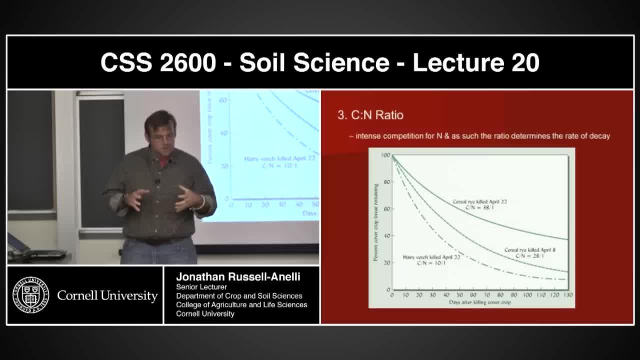 the nutrients in the system. We haven't really talked about this yet, but if you start thinking about nutrients, there are some nutrients that we need more of than others, right? I mean, if you think about sort of biomasses, we always have this. 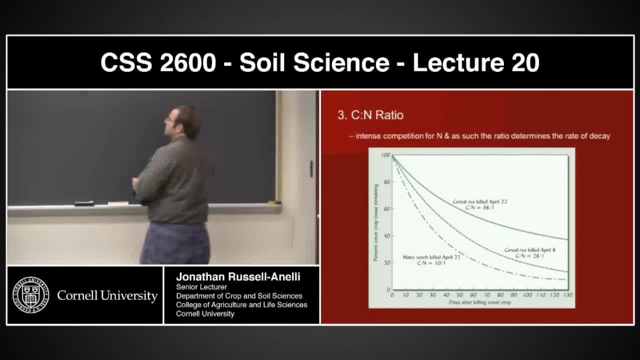 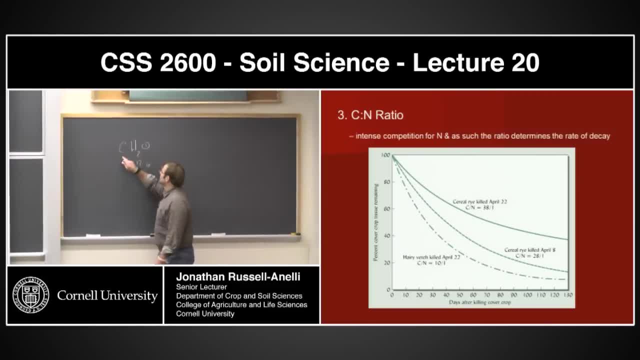 we always sort of give this really simple equation, you know, of what organic matter is and it's like CH2O, or sometimes it's 6,, 12,, 6, but we always sort of talk about these nutrients but we don't talk about the other macro and micronutrients. 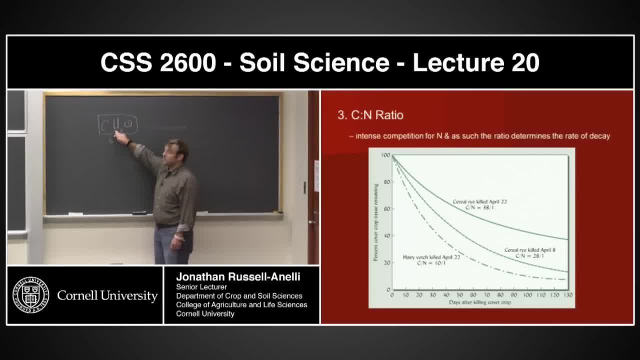 But if you're thinking about decomposition rates, you really have to start thinking about what's here, as well as all these other things, because when we're eating stuff, we're eating things for two reasons. One is we're eating it for energy. 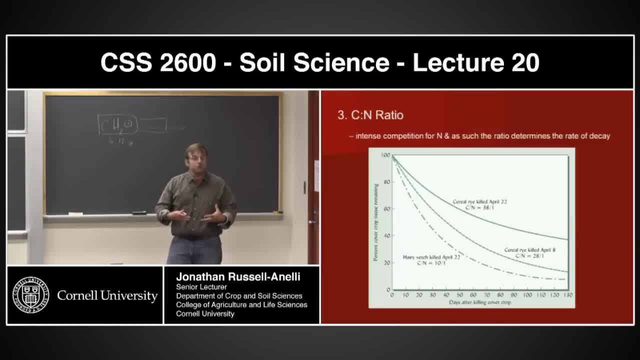 but the second reason that we're eating this stuff is we're eating it for nutrients. okay, Certain types of material have better nutrients, nutrient quality than others. okay, So you can certainly imagine that the nature of this ratio of carbon to nitrogen. 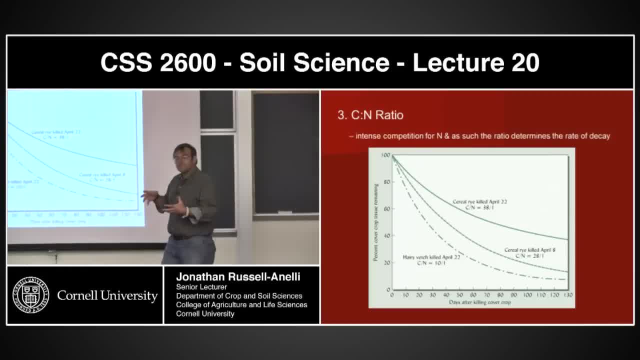 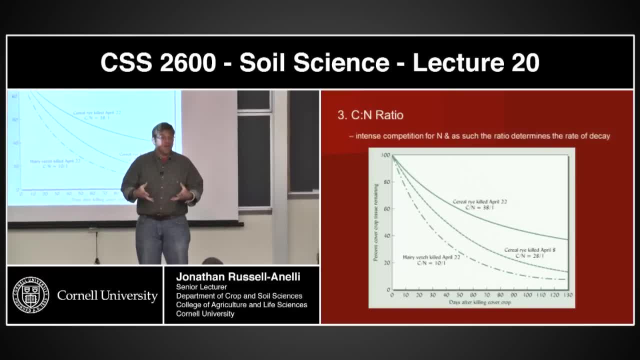 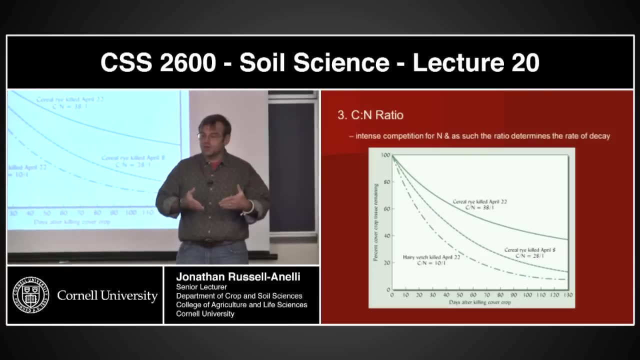 okay will certainly affect how readily this material is going to be acted upon, how readily it's going to be targeted to be eaten, And there is intense competition for these other nutrients. So CN ratio is a good sort of good example, because it could certainly easily be carbon-phosphorus ratios. 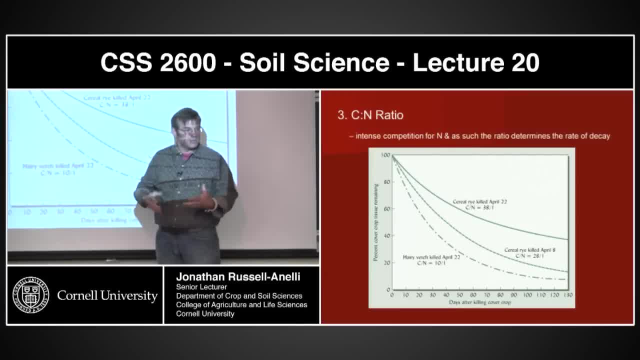 or carbon-potassium ratios, but nitrogen happens to be a very good example of what all these other nutrients are doing, and the ratio between carbon and nitrogen is a good reflection of how readily this material, the food material, is packed with nutrients. 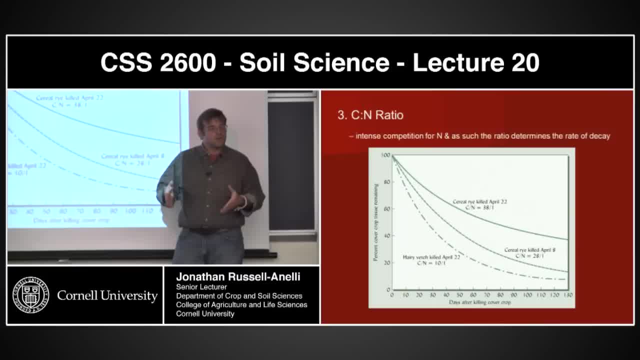 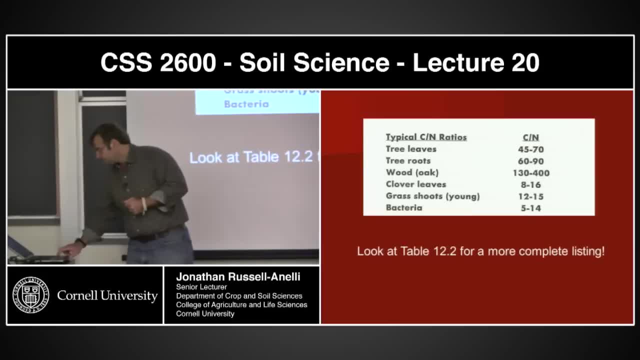 Make sense. Okay, there is intense competition for these nutrients. Okay, you've heard of woody type of materials and things like that. Actually, let me go to that slide right. Okay, these are the typical CN ratios of a lot of different types of materials. okay, Tree leaves, tree roots, wood oak bacteria as well as grass shoots. So the CN ratios of these. basically, if I have a wood or an oak material, I've got 130 to 400 carbons per one nitrogen. Does that make sense? 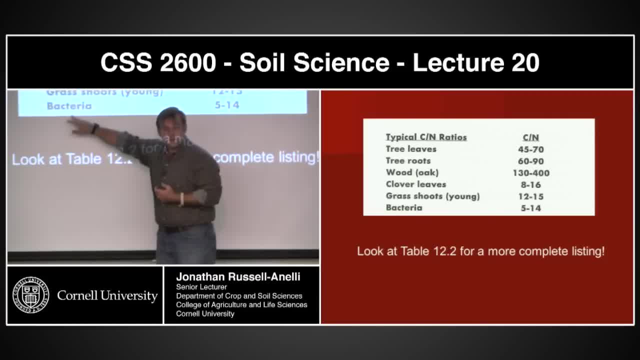 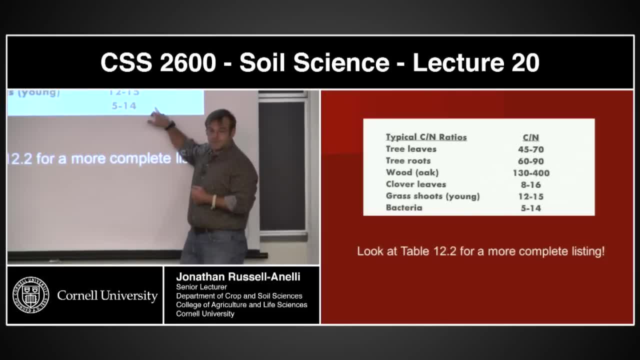 Okay, now look at the bacterial number here. The ratio of the biomass of a bacteria is five to 14 to one. So that basically says to you: hey, just from a biomass perspective, just from an organism's perspective, this organism has to have so much more nitrogen. 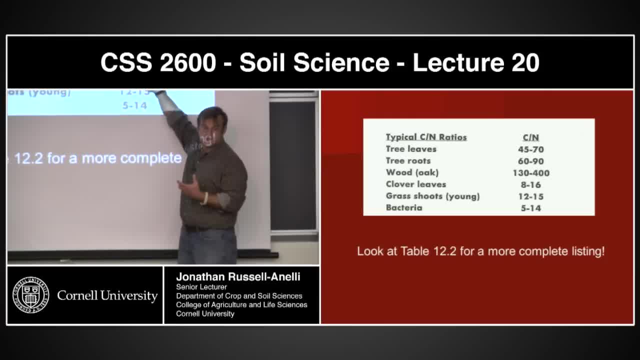 compared to its feedstock than carbon. Does that make sense? And so, as a result, the lower. as a result, the nitrogen is really in demand, because it needs to have a lot of that. Okay, now another thing that we often don't think about. 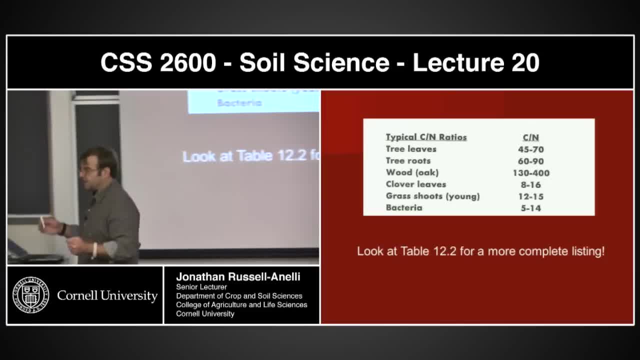 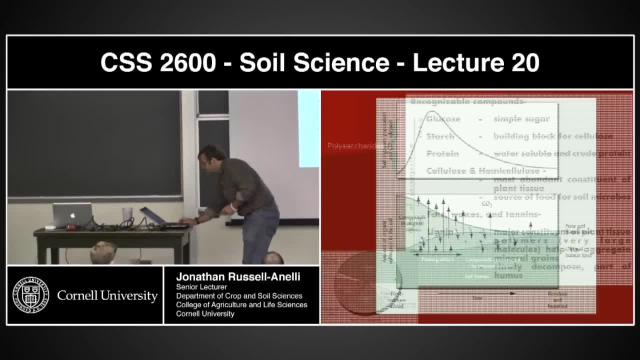 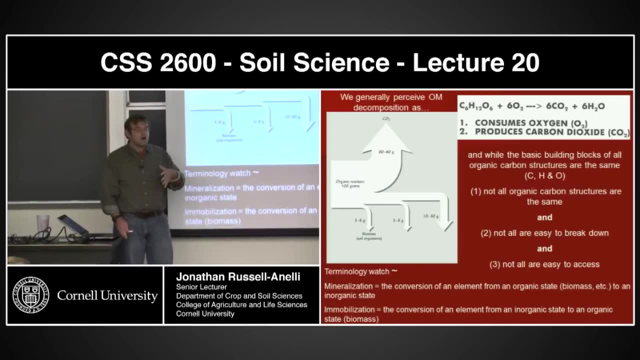 when we think about decomposition- and this actually goes to a slide that we showed before- The slide looks just show, show. I can find it quickly- This slide right here, this image right here. When we think of decomposition, we often think: 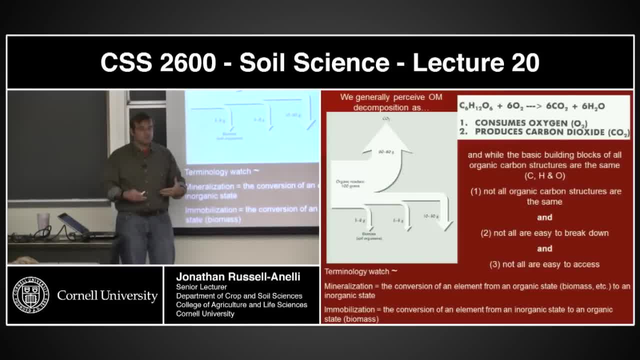 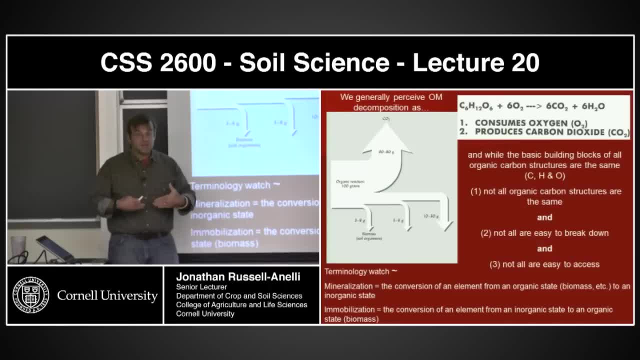 and I just said it to you guys right now: when we eat, why do we eat? We eat for energy and for nutrients, right, But in that process we eat for energy, But in the process of eating there's a lot of byproducts. 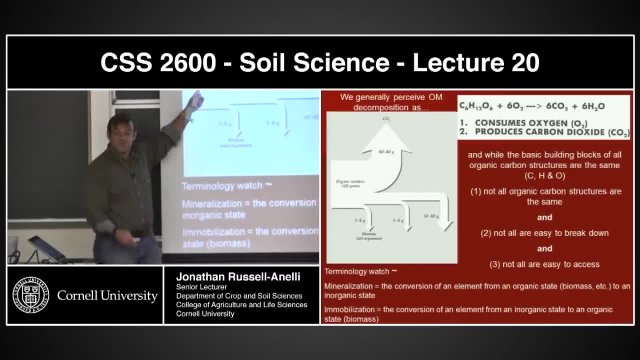 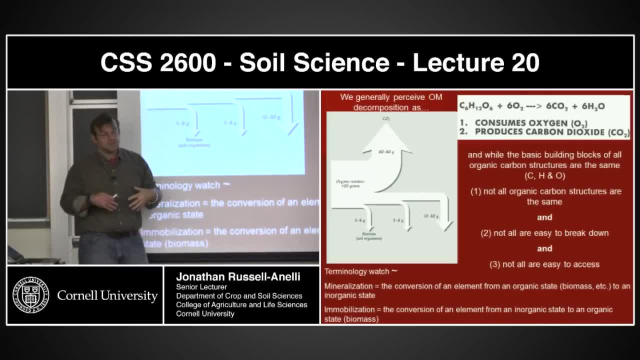 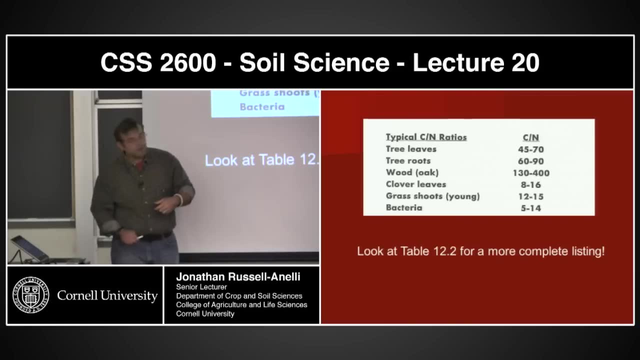 60 to 80% of this material, this 100 grams of material that I'm eating- is being blown off as CO2. So I don't get to use it in my biomass. So when you start thinking about- sorry, When you start thinking about these types of CN ratios, 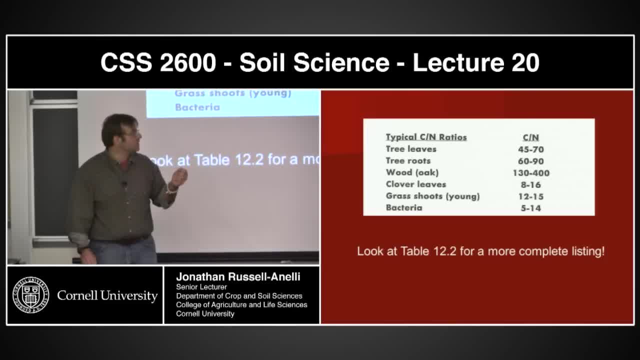 you also have to think about what's the byproduct of here, Because they're not. you're not going to get 100% conversion of this material. Does that make sense? Okay, now, if they were getting? this is not possible. 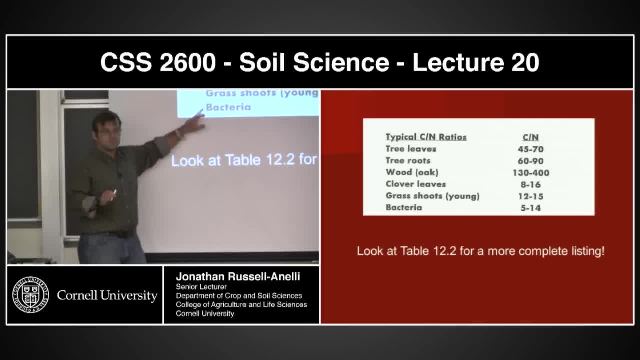 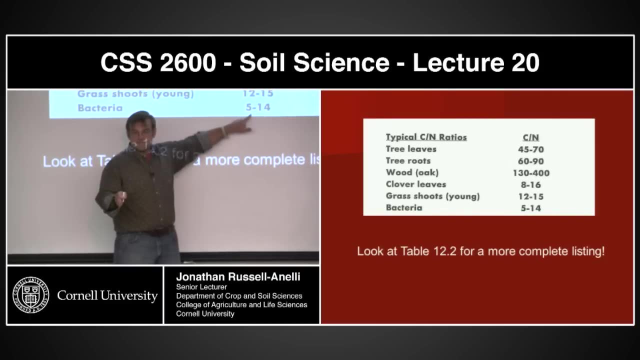 but if they were getting 100% conversion, the biomass, the CN ratio of the material that they want to eat, would basically reflect their body. Does that make sense? Questions about that Go Okay. if there was no waste whatsoever, everything I ate got perfectly used by my body. 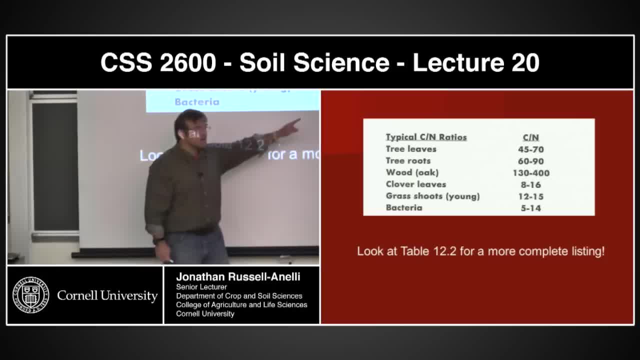 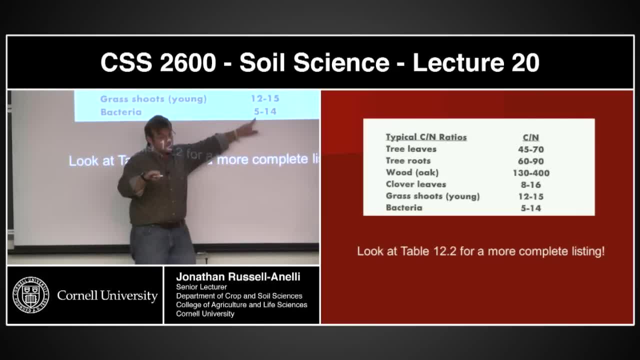 which it does. I might add: okay, But if I was a microbe, the perfect food for me would be without any kind of waste, would be 15 or 14,, five to 14 to one, because I would be eating what reflects. 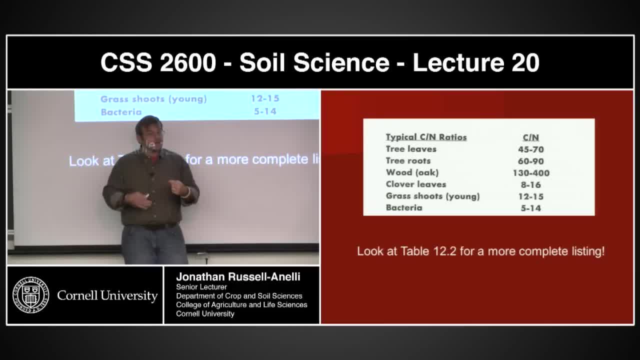 reflected my body. Now, the problem with that is that I need two other things. Well, one I don't need and one I do need. One is I need to get energy too, okay, And that energy is not reflected by this biomass. 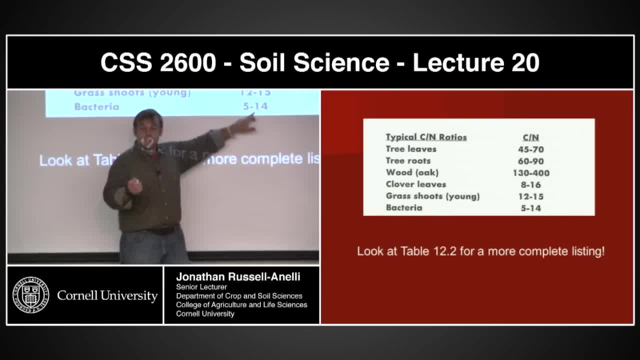 So, right there, the carbon-nitrogen ratio of my food stock has to be larger than my body, because I need to get energy too. And then, on top of that, I'm respiring and I have CO2 waste, which tells me that my ratio has to be even higher than that. 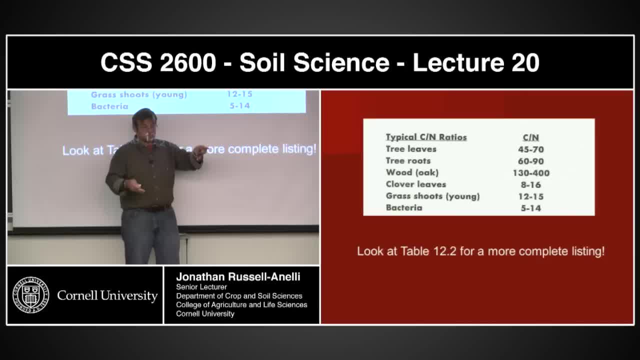 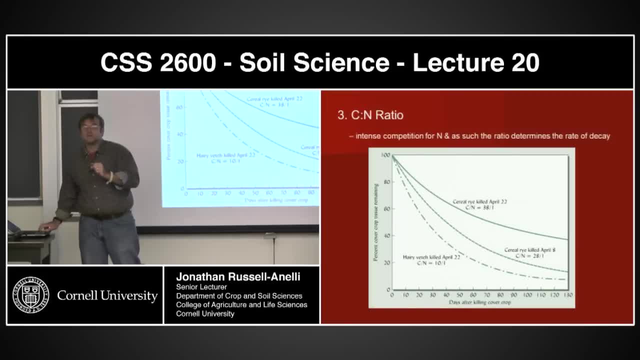 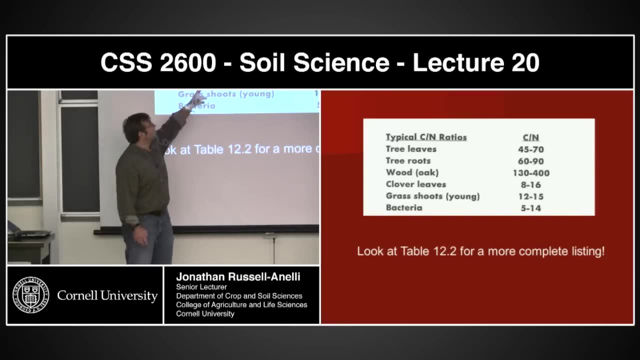 Does that make sense to everybody? Does that make sense? Okay, we good with this, So let's go what Go? How is biomass like? what does biomass have to do with these ratios? Well, different types of biomass. 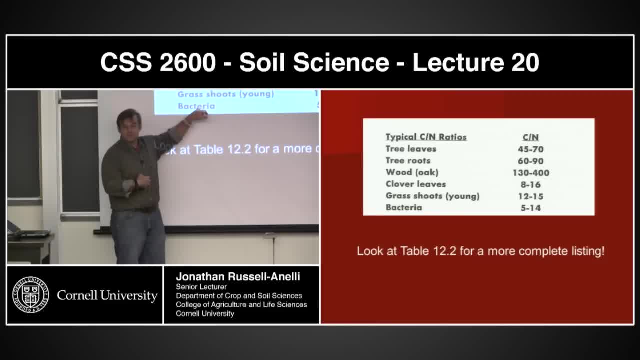 the food that you're eating versus the biomass of the organism. Well, different types of biomass- the food that you're eating versus the biomass of the organism. Well, different types of biomass: the food that you're eating versus the biomass of the organism. 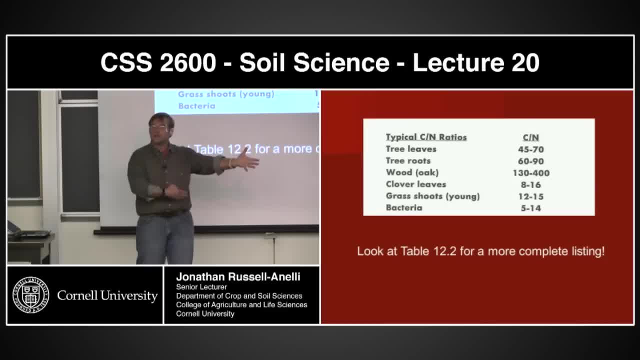 Have different CN ratios, because I mean, think about your body, My bone versus my muscle have very different CN ratios, Like that they're composed of different CN ratios. They're composed the particle itself, my nails, my hair, my eyes. 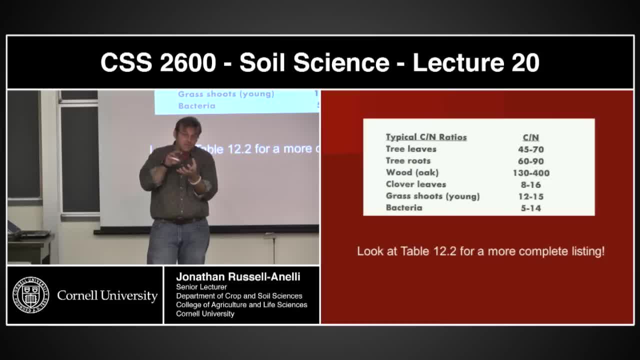 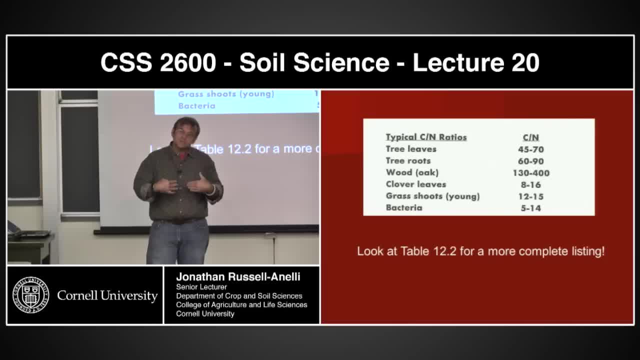 So when I die- which we all will- when I die, I'm gonna start decomposing. The organisms that are gonna be decomposing me are going to have different types of feedstock associated with my body. Well, the same thing's gonna go. 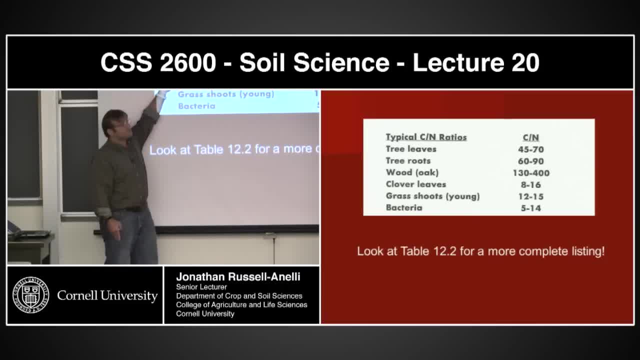 with all these other types of material. Okay, A tree is made up of a lot of different parts. It's got leaves, it's got roots, it's got bark, it's got cambium, it's got heartwood- All of those different components. 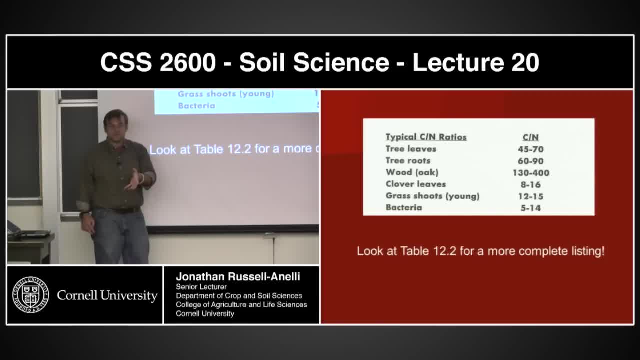 are gonna have different types of CN ratios. Okay, does that make sense? Which means that they are gonna have different combinations of C to N relative to this organism, Right, Okay, so let's write up here the things that the organisms are getting from decomposition. 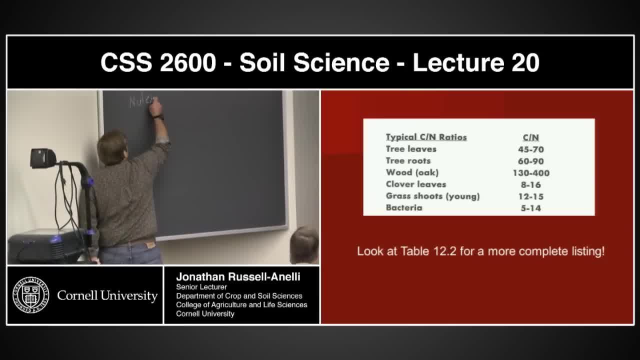 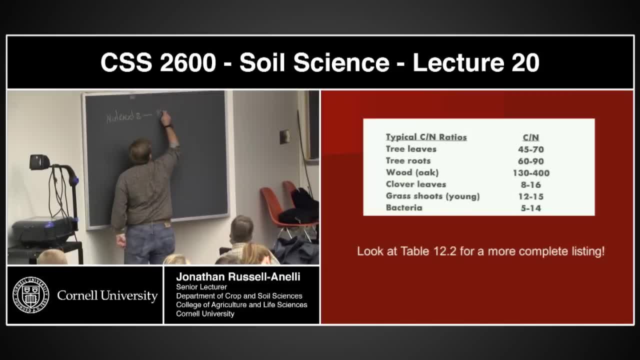 They're gonna get nutrients. Okay, in the sense we can say, this is they're building their bodies, This is biomass, right? Okay, they're also gonna be getting energy, You know, ATP, in essence, The other thing they're gonna do. 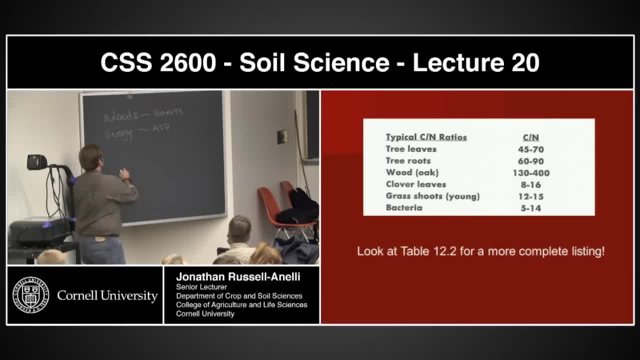 is they're gonna be producing waste, Right? Okay, so waste waste certainly is going to be material that they didn't actually digest, so it's gonna be waste food. okay, So more organic matter, just in a different form. 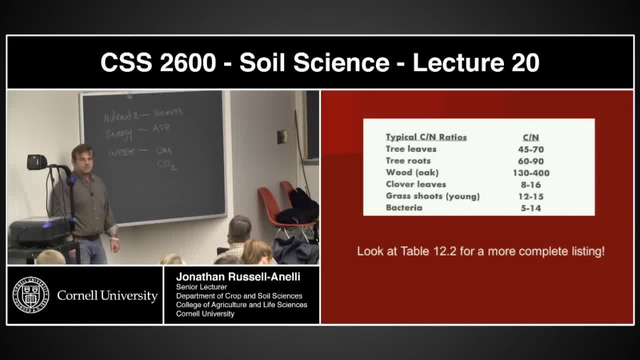 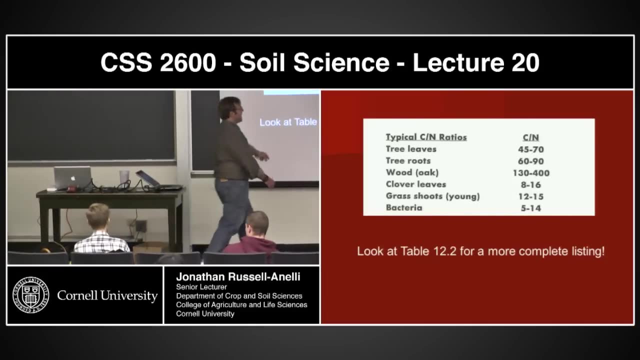 but they're also gonna be waste in the issue of CO2.. Right, Each one of these represents some of the material that's in that CN ratio. So if my biomass happens to be- let's make it simple- my biomass happens to be 10,. 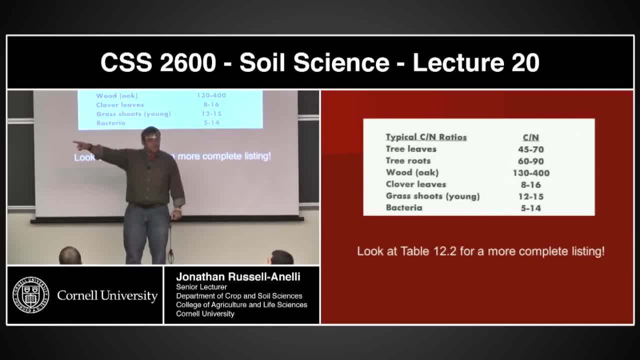 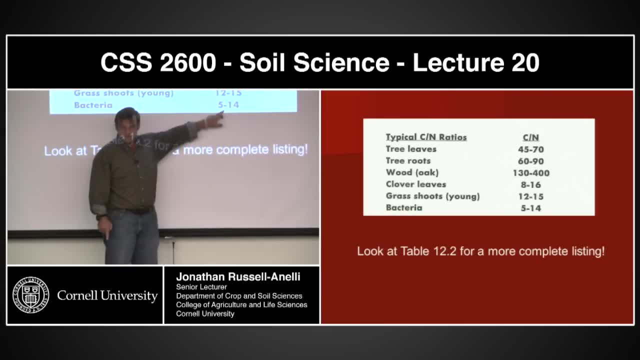 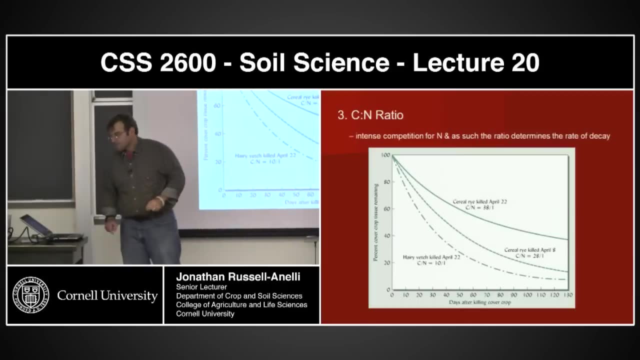 10 to one CN ratio. Look at all the carbon and nitrogen I need to be able to get to get to that number Right. Does that make sense? Kind of? Okay, let's take a look right here Now. this is gonna reflect two things. 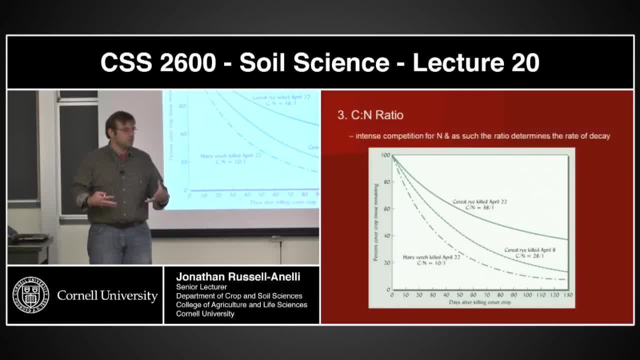 One is it's gonna reflect the speed of which things get decomposed And two is it's going to reflect- for lack of a better word- the selectivity of what's gonna get decomposed. Okay, what is gonna be targeted and how long is it gonna take to decompose? 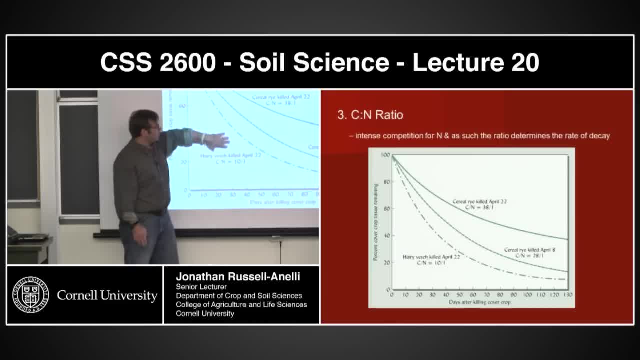 Okay. so right here I've got three different, three different models. well, actually, two of them are cereal rye and one of them is a hairy vetch. okay, they were killed at different times and they have different CN ratios. okay, and what you're looking at here is the percent crop remaining. so as it goes, down, it's being decomposed and this is time, okay. this is time from the kill, okay, or time from the addition. okay. cereal rye: here's a 38 to 1 CN ratio versus hairy vetch, which is a 10 to 1 ratio, which one gets decomposed faster the 10. 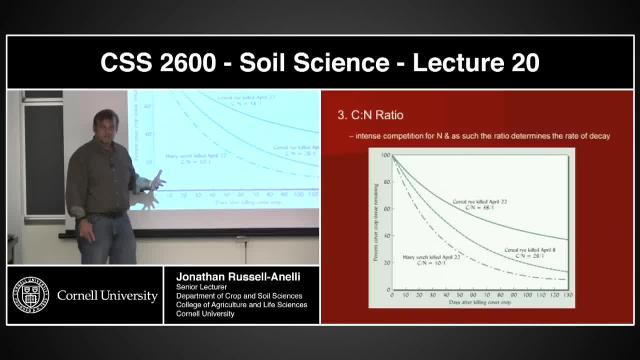 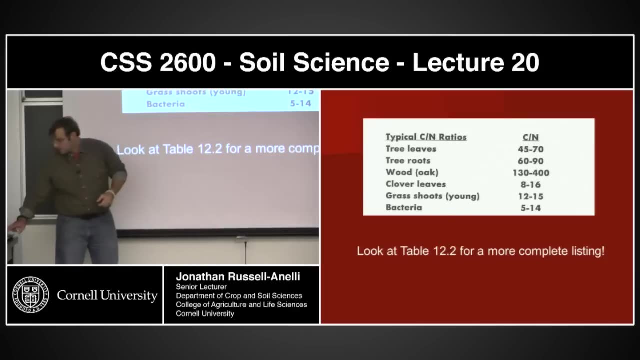 to 1. well, why some more nutrients have packed into it. and of my selectivity is I really? there's a lot of competition for this because, look look at this, most of this material has really high CN ratios. oops, wrong way. this has got a 10. 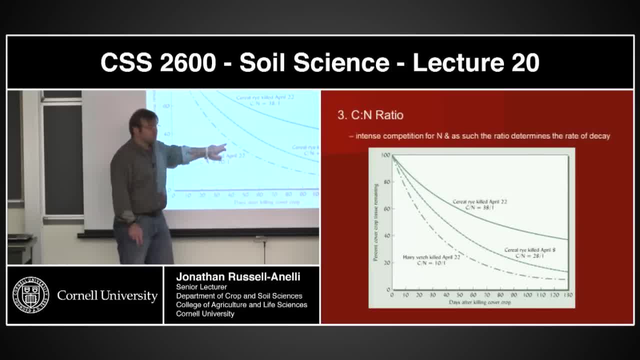 to 1. this has got a 38 to 1 and so, as a result, this stuff gets decomposed faster, just at CN ratio go. is the CN ratio correlated to what degree of lignification? no, because I can't use my body in this case. we don't have a lot of. 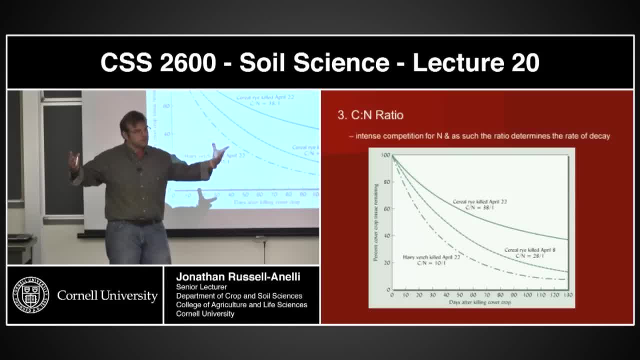 lignin. but if a plant, if you look at the plant tissue itself, in fact, lignin actually tends to have dropped, the CN ratios tend to be lower. but having said that, the many of these materials, lignin as a decomposes, actually the CN ratio gets lower and lower and lower. okay, so it's, it's not. 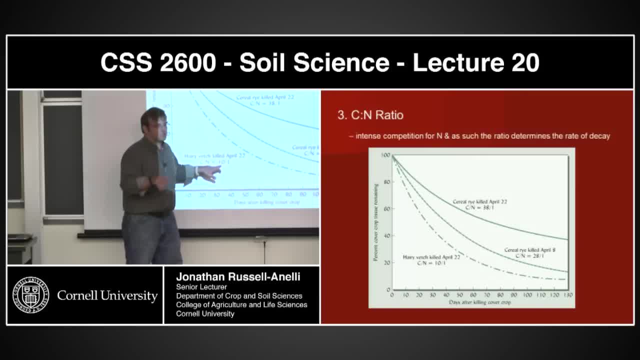 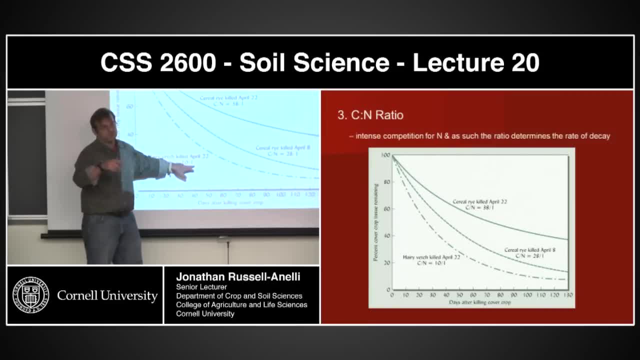 necessarily a measure of its, a measure of the material. now, as it decomposes, this CN ratio will change and that might be a better measurement of lignification. does that make sense? ok, so we have these two different materials: high CN ratio, low CN ratio. the high CN ratio is a lot slower to 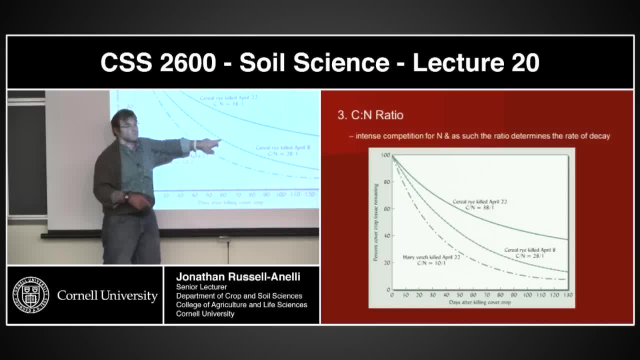 decompose and in fact if you take the same material you just kill it at different dates. the CN ratio has changed, so it's not necessarily nature of the plant. this is a 38 to 1. this is a 28 to 1. the 28 to 1 is decomposing a lot. 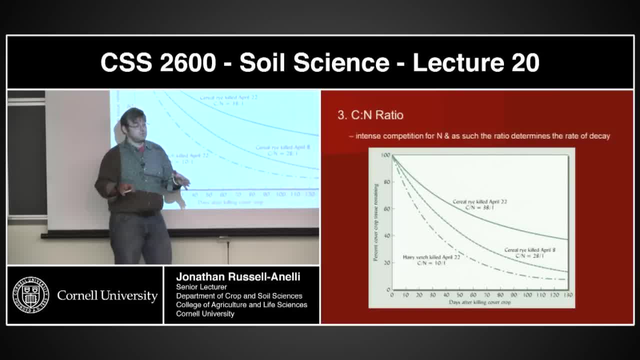 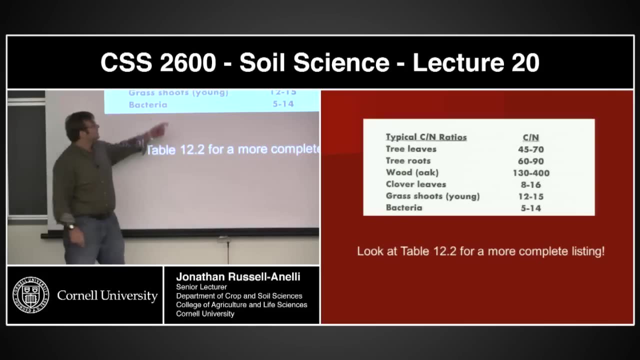 faster than 38 to 1. okay, just the ratio. okay, now that decomposition reflects this issue of what they're going to be using it for- biomass energy and these waste products. okay, and that decomposition is going to be reflected in those CN ratios. okay, now I need to stop here because I want to make sure. 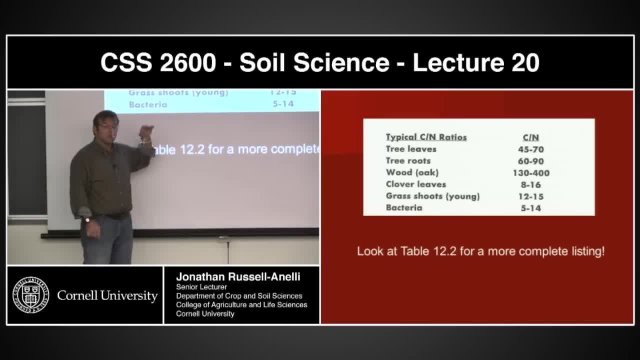 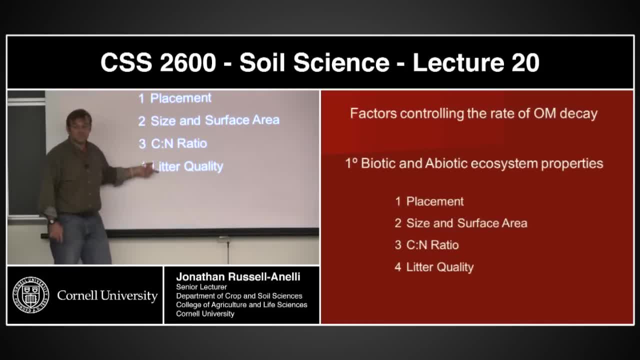 everybody understands that this is just CN ratio is just one of all four of all four of these controls on decomposition. this is just happens to be one size and surface area happens to be one. the reality is, all of these are in combination. this one happens to be the. 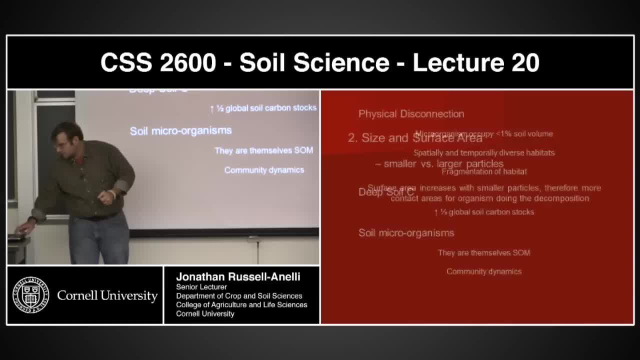 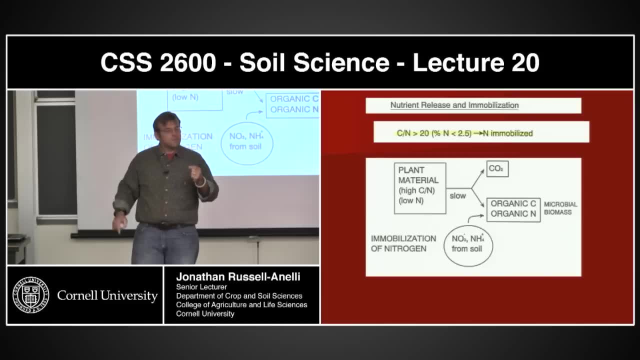 most important. okay, so let's keep going with CN ratio, because I don't want you to now. it turns out, because of this issue over here, that the magic number- if you think about this, the magic number of carbon nitrogen for decomposition, tends to be around 20. okay, 20 to 1. okay. now, what do I mean by that when the CN ratio? 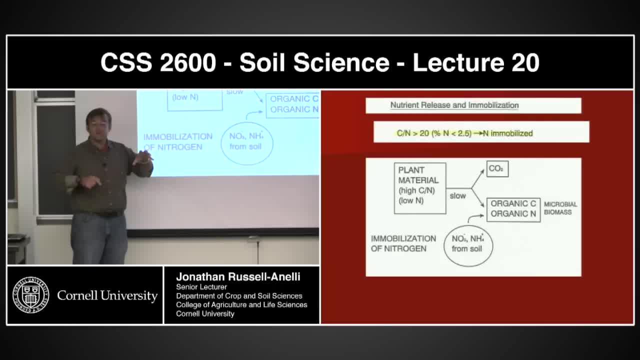 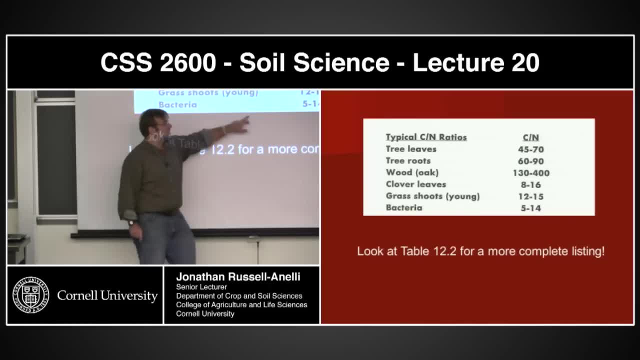 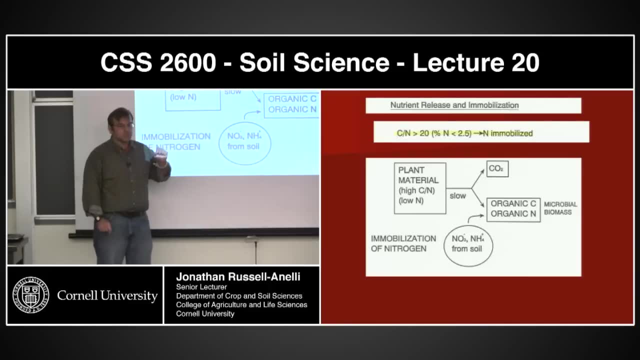 is greater than 20 to 1. I got a lot of carbon, very little nitrogen because of the organisms that are doing the decomposition, mostly these guys and their CN ratio. because of that ratio, most of the nitrogen is going to be immobilized from that decomposition. remember what immobilization means? basically, I'm taking a mineral form and 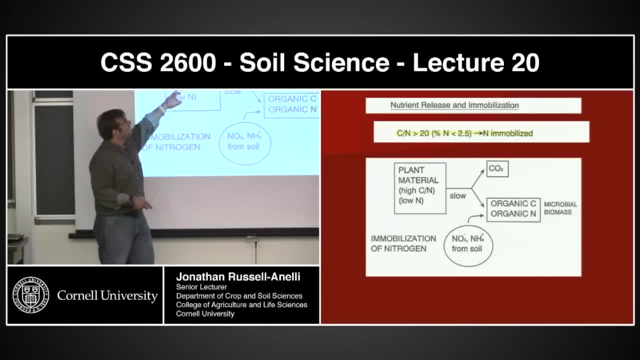 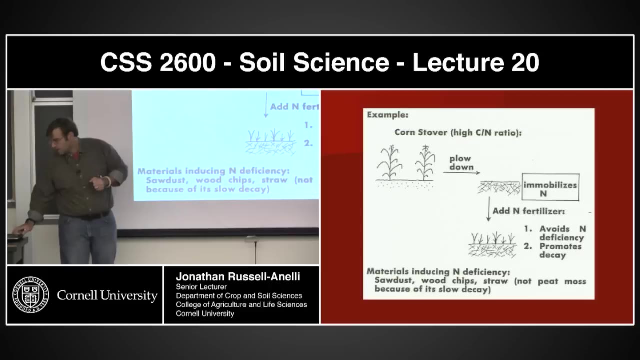 turning into an organic form. okay, so the nitrogen that is in this plant material, greater than 20 to 1 to one, the nitrogen that's in this plant material is basically being taken up by the organisms that are doing the decomposition. Now that ratio has to do with that biomass, ATP and waste. 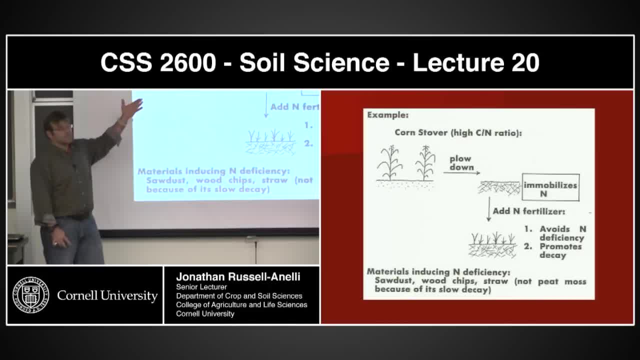 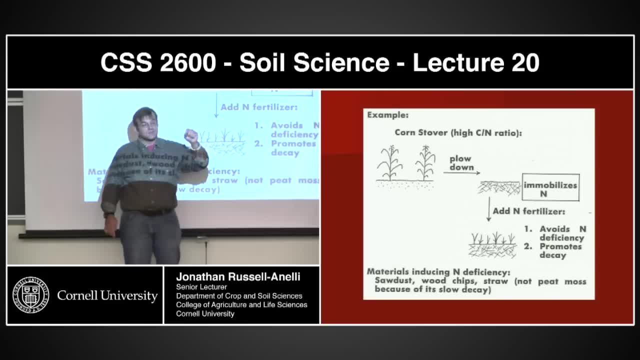 Good examples are this, or something like a corn stover where I have a high CN ratio. I plow it down. it gets into the soil. The nitrogen that's in that soil basically get immobilized, In fact the organisms that are there, if the nitrogen isn't actually in the organic. 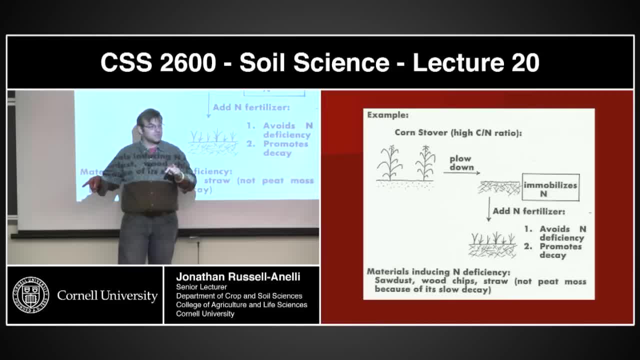 matter that they're decomposing, they'll take nitrogen from other sources, because this represents energy as well. If they can get the energy and they can get nitrogen from another source, they'll take it. As a result, we often have issues of nitrogen deficiency when we add high CN ratio material. 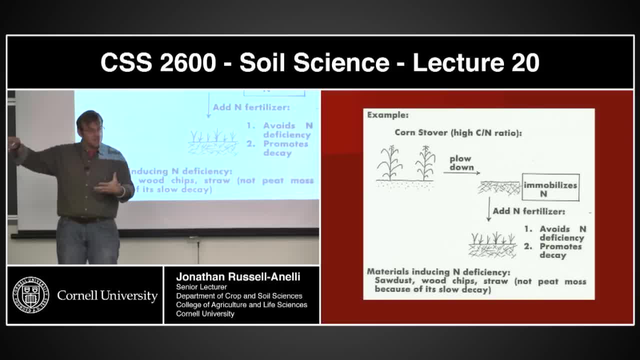 because the organisms are much better than the plants at getting nitrogen. They can move around. As a result, they'll start harvesting nitrogen from other sources, because they're all about that biomass. It turns out that this is usually a very temporary effect, but it depends upon the type of material. 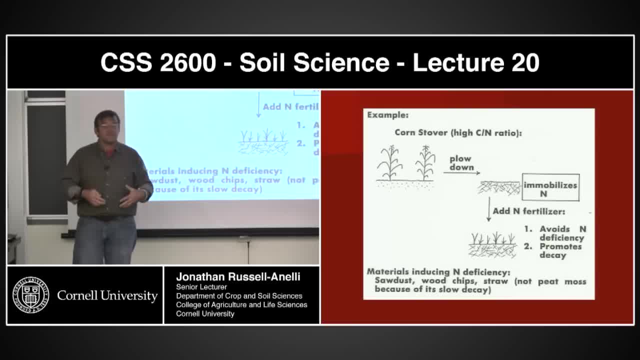 that you're using, If I have a high CN ratio material that is really slow to decompose, like a wood chip type of material. the organic matter takes a while to decompose so that nitrogen deficiency is attenuated. It's slowed up. 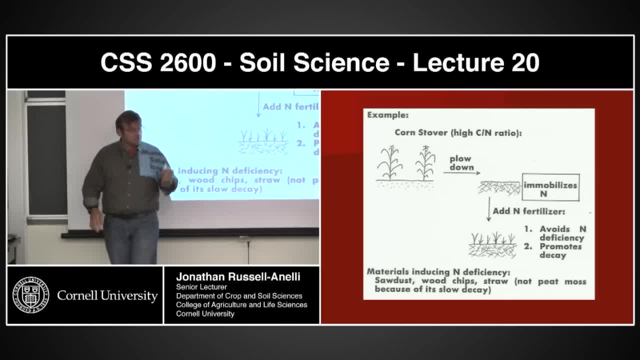 It's not as dramatic. On the other hand, if it's a straw that decomposes very easily, that's when you're going to start seeing the nitrogen being taken from other sources. As a result, you'll get that nitrogen deficiency. The reality is, though, that these nitrogen deficiencies are relatively short term, because 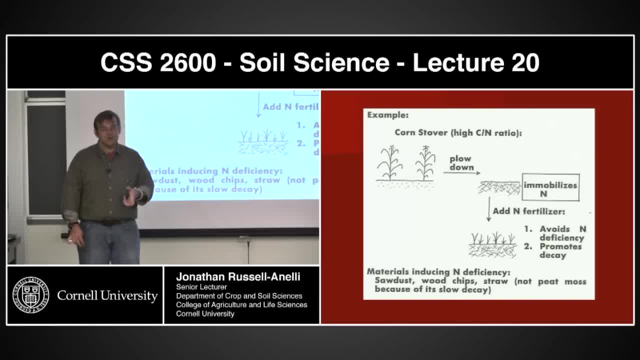 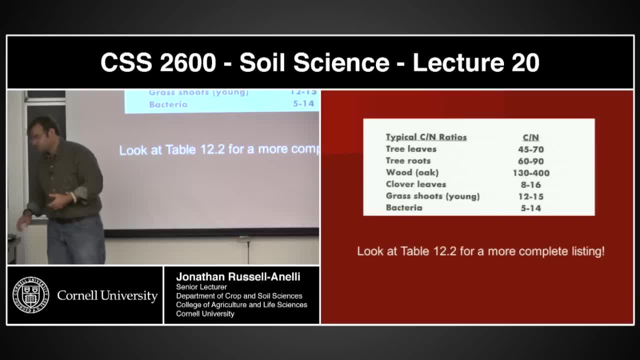 what's going to happen to these organisms? they, in turn, are going to die. When they die, they'll release the nitrogen again. Does that make sense? What is their CN ratio? Basically, they've been concentrating the nitrogen and when they die they become a. 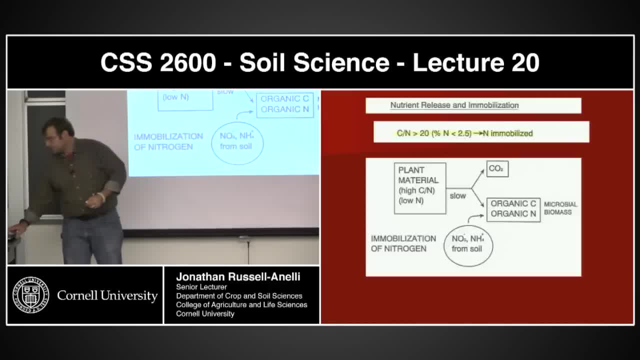 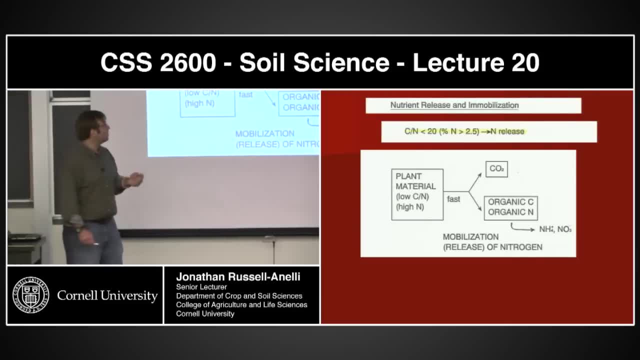 low CN ratio material, which leads us right into this next number. When the CN ratio is lower than 20, generally, the nitrogen gets mineralized, It gets mobilized, It gets released. If you're putting in material that has a low CN ratio, you're basically acting. you're. 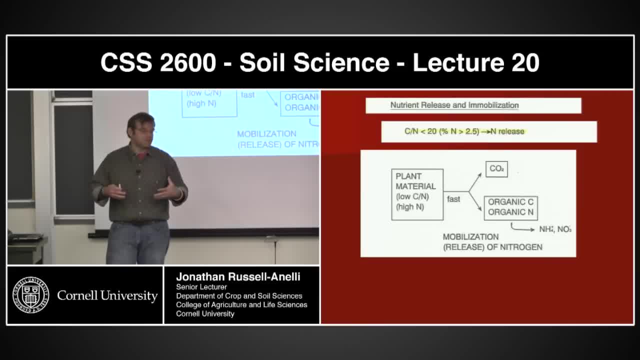 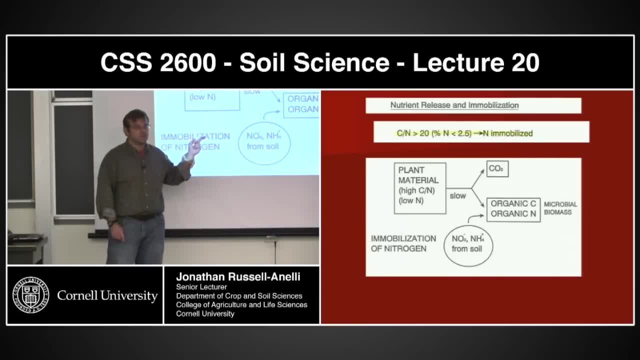 basically fertilizing. It still has to decompose, but it's a quick fertilization compared to the slower fertilization that's associated with a 20 to 1.. Does that make sense to everybody? Questions about that Go. Have they correlated the time of decomposition with nutrient release? 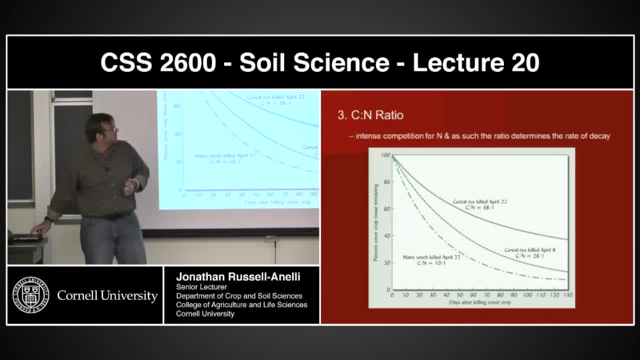 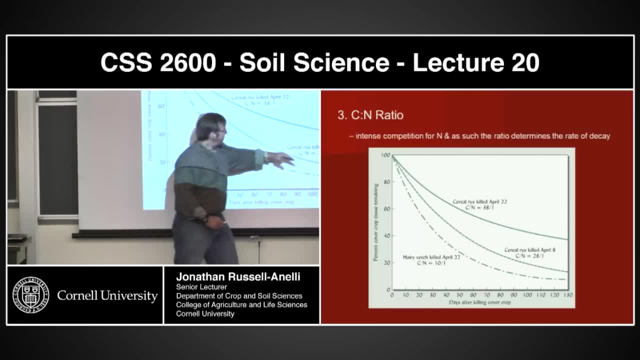 Have they incorporated the time of nutrient release on this, If we go back to a slide like this? yes, they have numbers that are associated with this. If you take a look at this material, yes, it's going into biomass, but if it's a 10. 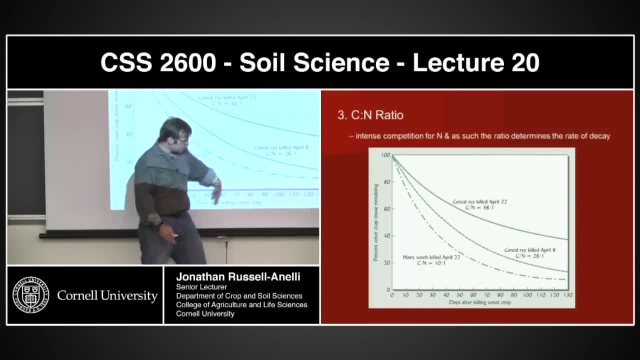 to 1,. this material is also releasing nutrients and the timeline right there is 130 days. Have they quantified that It depends on the type of material and the type of environment you are in? but yes, Did everybody hear that question? 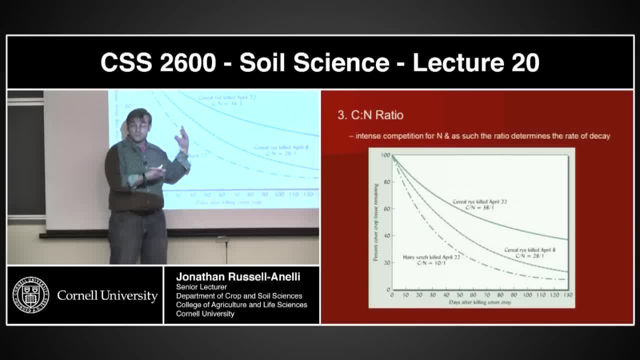 Do they have an idea about how much nitrogen or fertility is actually going to be released through decomposition? Yes, They have, because basically, what you can do is you can take a look at these numbers and you know how much is going into biomass. You can predict how much is coming out as fertility. 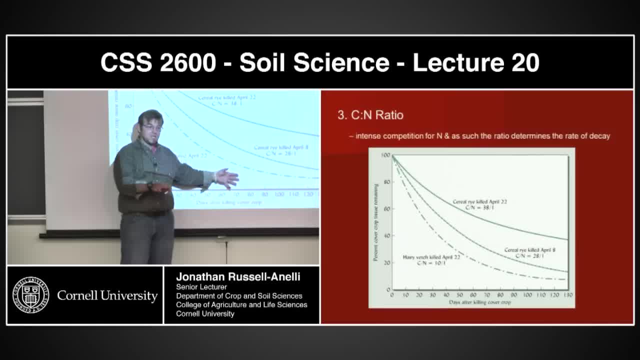 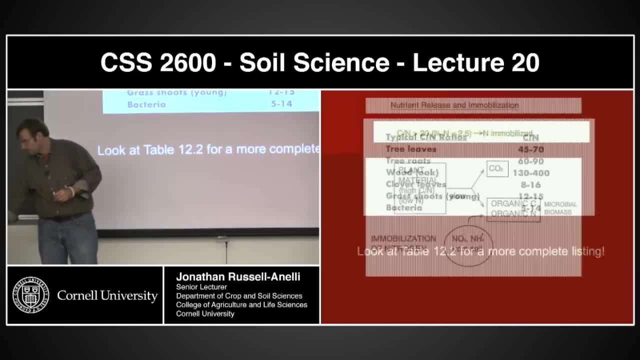 Now that doesn't necessarily mean it's going to be making it to the plants, but it does mean it's going to be released. Question: You said that nitrogen will get immobilized with a high C to N ratio for short term. What would you classify as short term? 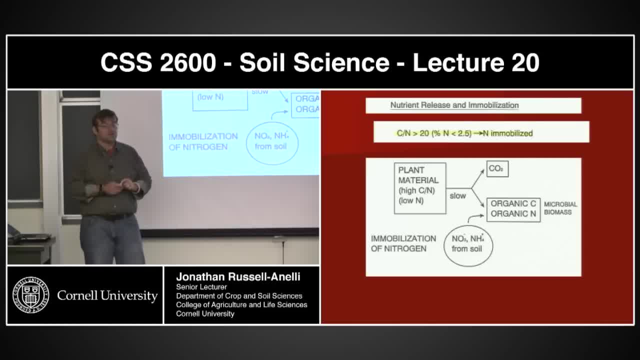 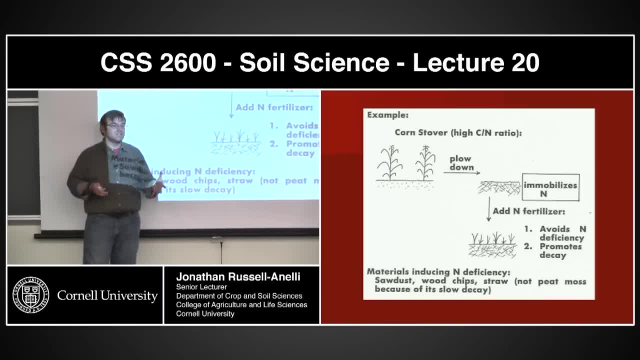 Okay, so the question was the nitrogen, and with a high C to N ratio, the nitrogen is going to be immobilized. Immobilized for a short period of time. What, in fact, is that period of time? I do not have an answer for that one. 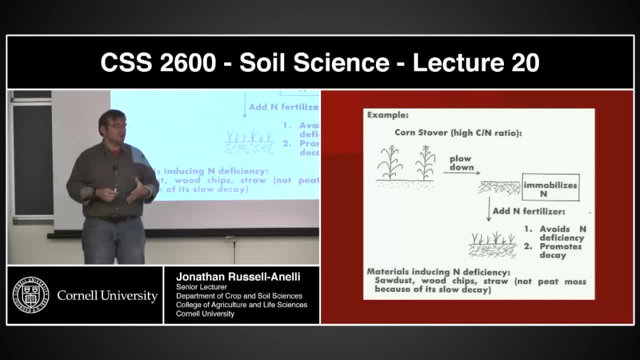 But in general. Oh. so how long are we going to have this nitrogen deficiency issue? You know, if it's in a garden, it's less than a season. I mean, if it's a lot of organic matter, it also is going to have to do with how much. 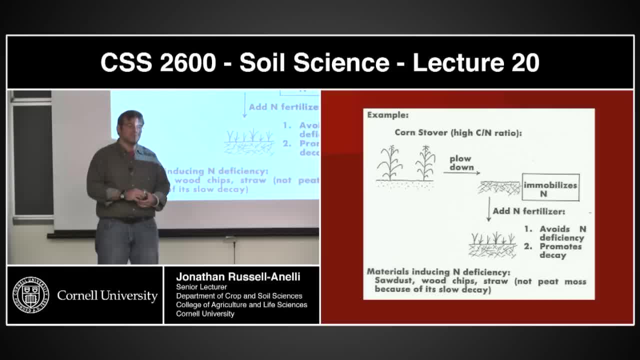 organic matter you add in, But it's not. It's not. It's often you see these garden magazines that the gray literature does. anybody read garden magazines? This is another. I'm just the only geek that does that. Okay, there's a lot of literature out there that says: you know if you add woody chips. 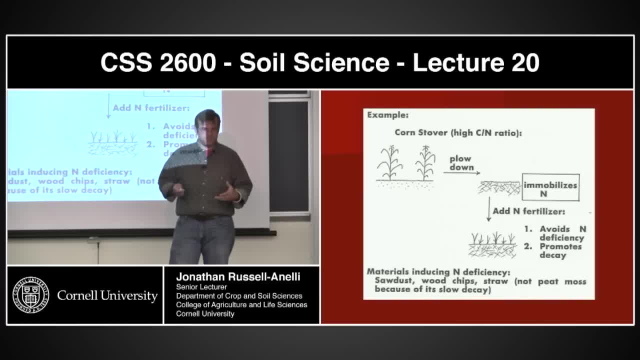 to your soils. you're basically you have to fertilize because your plants are going to be hit because they're not going to have any nitrogen. Well, it's not necessarily true. It's usually a localized effect. Okay, so if I put woody chips up here, my localized nitrogen deficiency is not going. 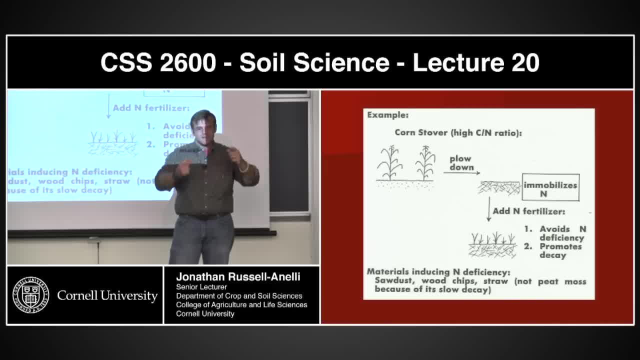 to be all the way down here, It's just going to be very local, okay So, and usually within the year, usually within the growing season, the plants are fine. Now, that's not to say that the plants themselves aren't going to be mining for nitrogen, as 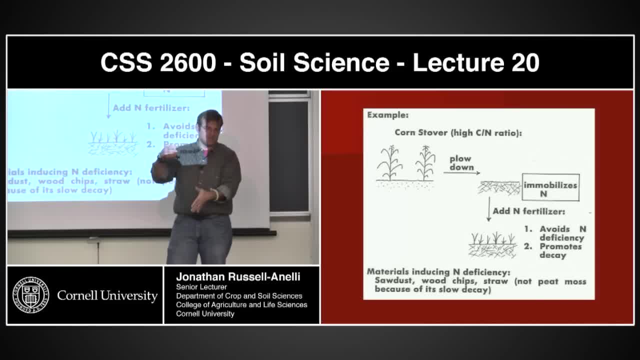 well. So that's not to say that if I put woody chips on the top I don't have to fertilize. I mean, if I put woody chips up here, I might actually be putting in some other types of organic matter that are going to decompose faster so they can provide nitrogen. 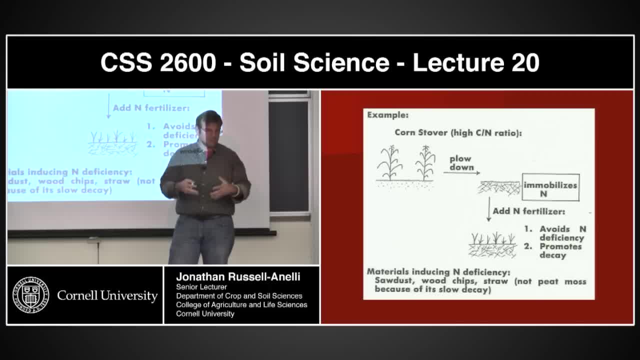 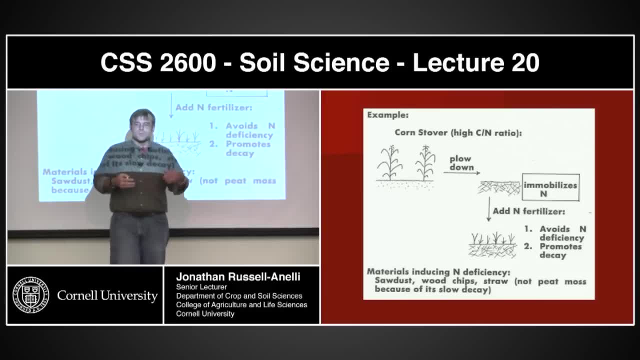 Because when those plants are in there, they're going to be sucking up nutrients, nitrogen being one of them. Does that make sense to everybody? So? so mulching shouldn't immobilize, Mulching should. when you mulch, mulching should not immobilize at any kind of rate. 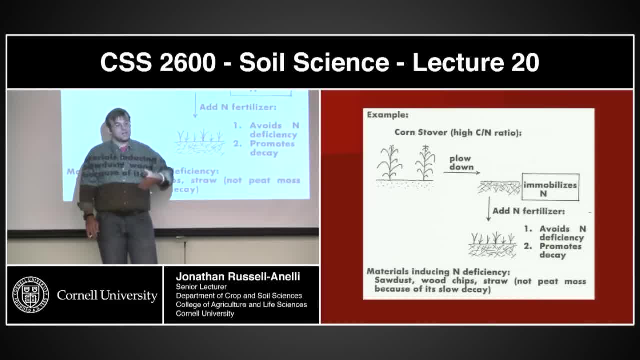 that is going to be problematic for plants. Now, when you start integrating that and that mulch starts to decompose and you start integrating and you put more mulch in there, yeah, you're going to have those localized temporary nitrogen deficiencies. But- and they do exist- 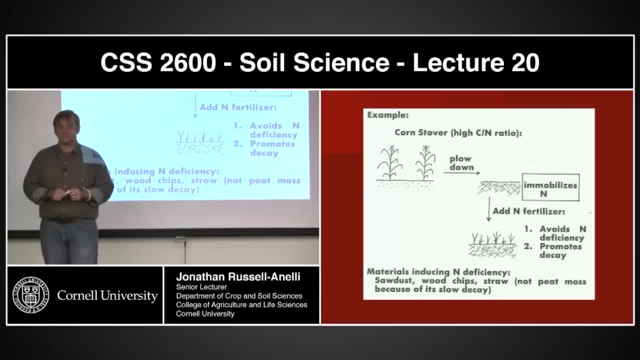 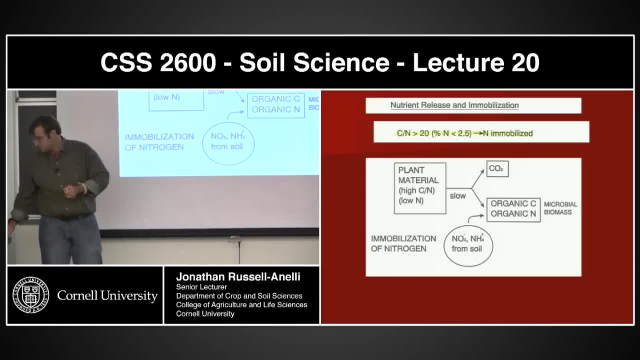 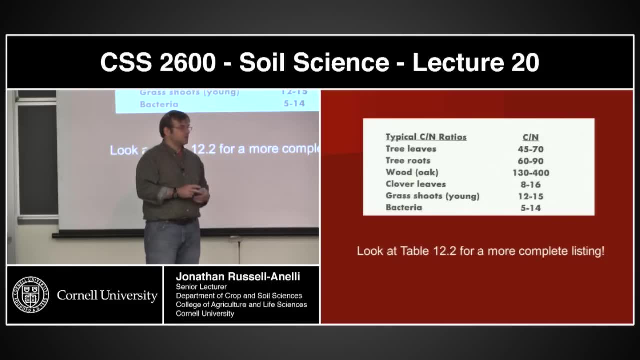 But if you're aware of them, you can manage for them. Okay, questions We good with this Go. Isn't it dependent on what kind, what CN ratio you in terms of what plants are growing? Okay, so the question is: doesn't it matter what kind of plants that you have in location? 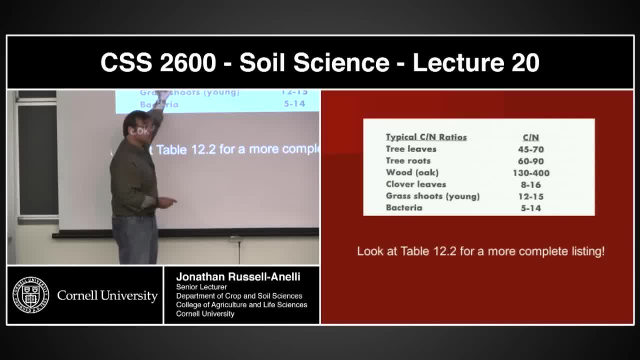 And yeah, that's definitely. that's definitely the case. It matters what kind of mulch you're using. it matters, I mean, I could put a allelopathic type up here too, but that has nothing to do with the CN ratio. 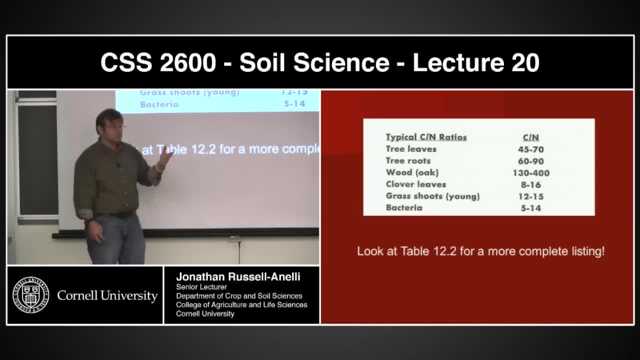 You know it depends on what I'm using for my mulch. I mean, there's grass mulches, there's wood chip mulches, there's all different kinds of mulches, And it also depends on the type of plant. You know, if I'm putting in, if they're young seedlings and things like that, that may be. more problematic than a more established azalea or rhododendron or something like that? Does that make sense? You know, if I'm putting in, if I'm putting in seeds into wood chips, one should expect you're going to have problems. 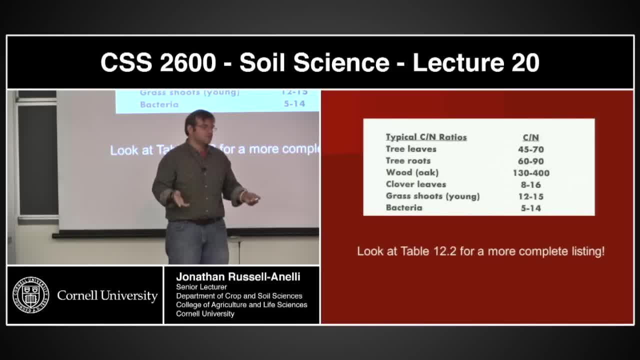 On the other hand, if I'm putting in seedlings or something like that, less of a problem. You know it's where those plants are trying to harvest their nutrients and if they're in that nitrogen deficiency zone, You should expect to see them having problems, because the microbes are much better at getting. 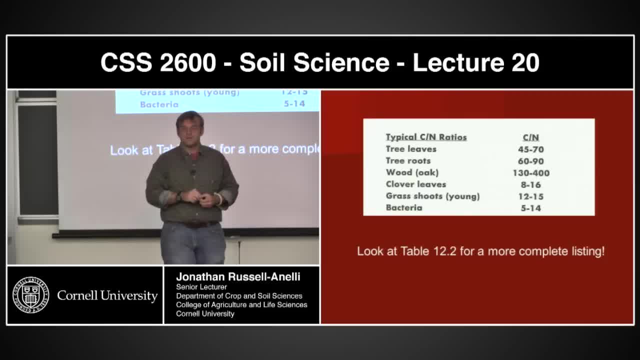 it than they are? Question: Yeah, like wood has a 130 to 400 carbon nitrogen ratio, so it would have a lot of nitrogen. No, it would not have a lot of nitrogen, it would have a lot of carbon, Carbon to nitrogen. 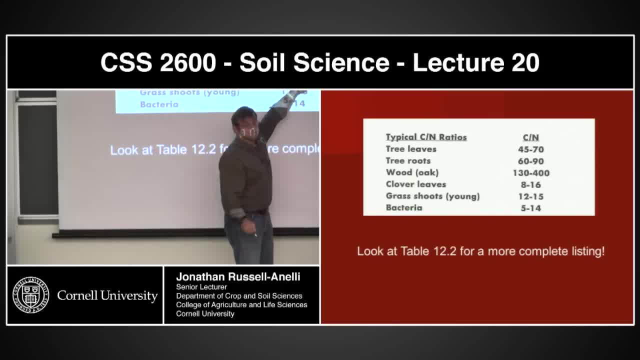 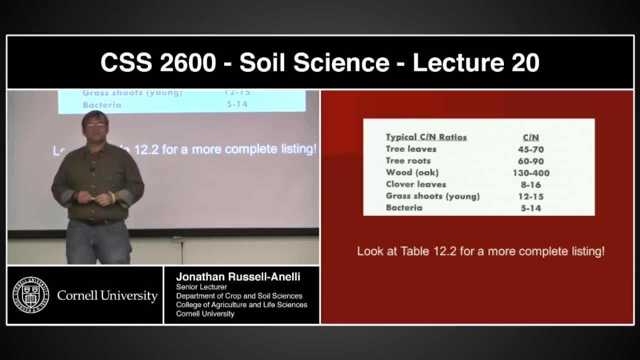 The first number is always carbon. so if this is 400, that's 400 carbon to 1 nitrogen. Oh, I thought that was 130.. Yeah, sorry, Could it matter how the organic matter is incorporated into the soil? So the question was: does it matter how the organic matter is incorporated into the soil? 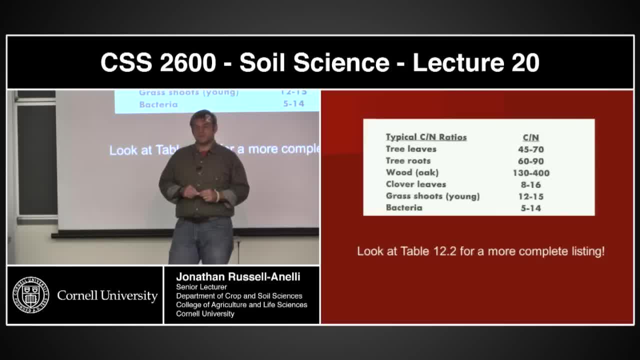 And often it does, but it's. that's a management decision. If you're putting all of your organic matter on the surface, that's going to be where the organic matter is going to be first reacting. You know. if you integrate it in, it's a different matter and you know. so we often use, we just 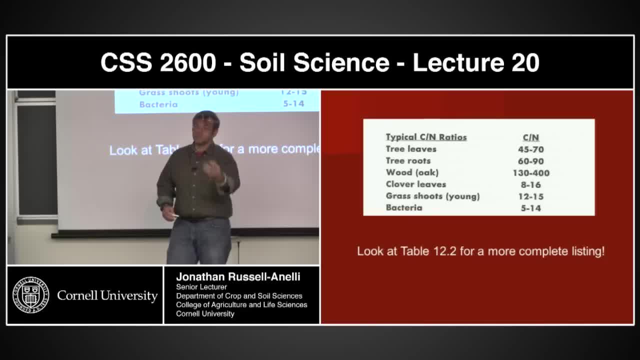 do organic matter on the top and let the organisms do the transportation. you know the worms will bring it down as they decompose. the material gets decomposed, it gets smaller and it will start moving down as well. The organisms themselves will move down there and they are part of this biomass as well. 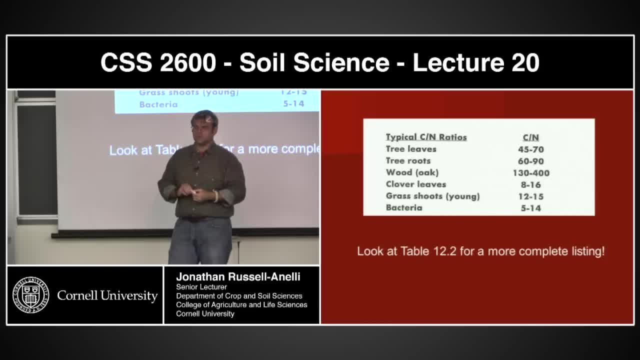 But it's really an issue of what you're trying to grow and what you're trying to you not necessarily grow, but what you're trying to do with that organic matter. Does that sort of answer that I'm not sure it does, but 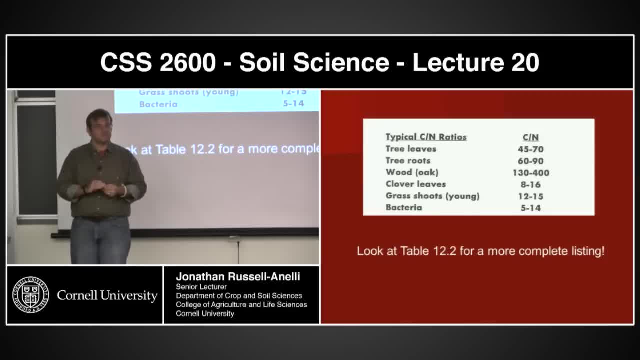 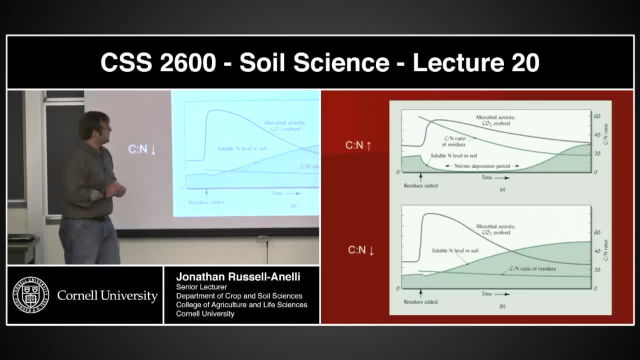 Okay, Any other questions on this one Do? we feel pretty comfortable with this, So I put this slide in here just sort of as a summary slide, and basically you have two different materials here. Up here is a high CN ratio, down here is a low CN ratio, and you've seen these graphs. 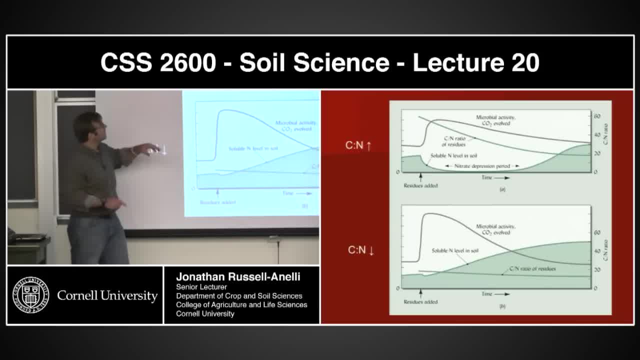 before. This is when I showed the CO2 evolution and decomposition. Okay, so this black line here up here and here is basically the CO2 evolution. Okay, Basically it represents the activity microbial community. Okay, It's their respiration. 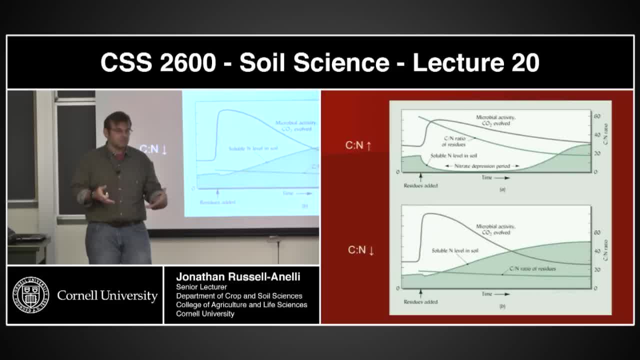 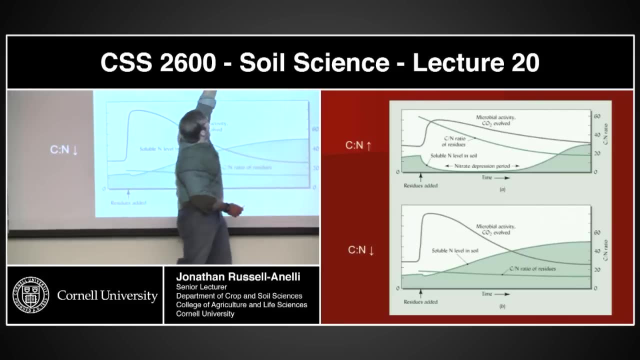 As it increases their pop the cop, the. the population is more active, Okay, And we usually associate that with a larger population. Okay, Granted, it could be one really large micro, but okay, The green line that you see there here, right here and right here, that's the CN ratio of 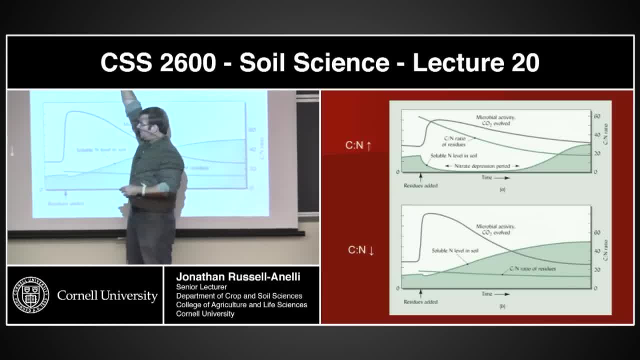 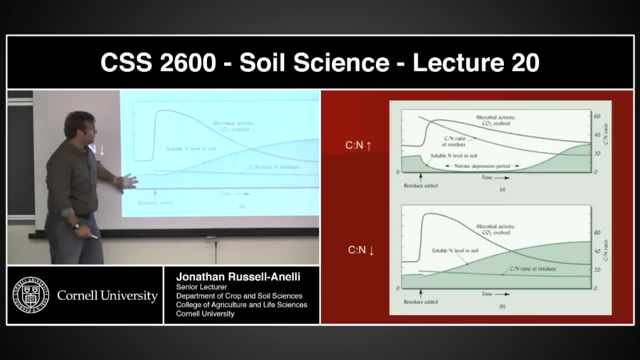 the material. So here it starts very high, here it starts fairly low. Okay, The green line that's underneath the green shade. that basically represents the amount of nitrogen that's released into the system. Okay, So as that nitrogen comes down, there's less nitrogen in the system. 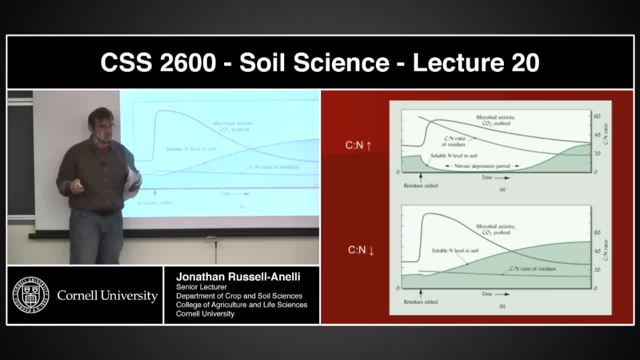 Now they're looking at nitrate, but nitrate is one form of nitrogen. Okay, As that number, as that line gets down, the available nitrogen in the system is depressed. As it goes up, the available nitrogen is increased, Right. 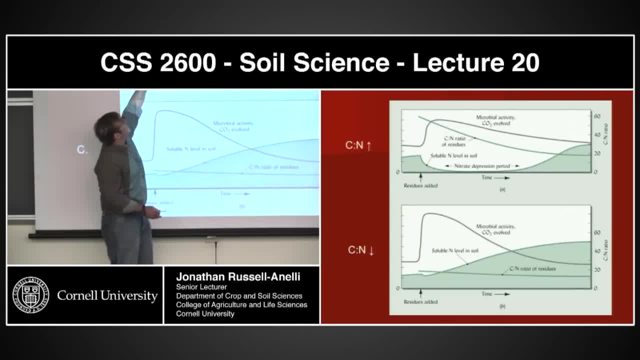 Okay. So if I start with a high CN ratio, Okay, Fresh added material. right here. you can see my population just boom, but you can also see my nitrate being depressed. Now this is the nitrate that's in the soil, not the nitrate that's in the nitrogen. that's. 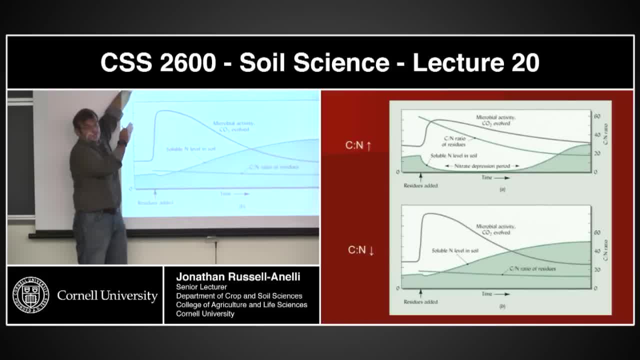 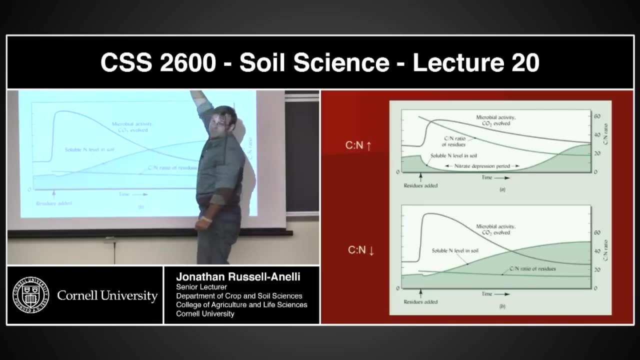 in the CN, not in the plant material that they're eating. Okay, So they're harvesting this nitrogen from someplace else. The soil, Okay. As time goes on, the population decreases, the CN ratio of the material also decreases and somewhere down the line, that nitrogen, that nitrogen that's in the soil, that's available. 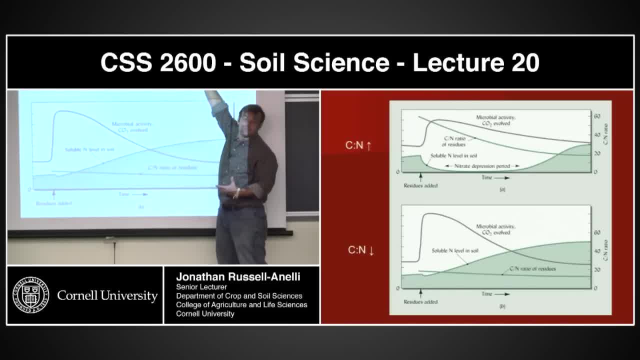 Okay, Nitrate, that's available. nitrogen starts to increase again. The populations are crashing. Okay, They're dying, They're releasing their nitrogen. On the other hand, low CN ratios, material population does the same. bop comes up. 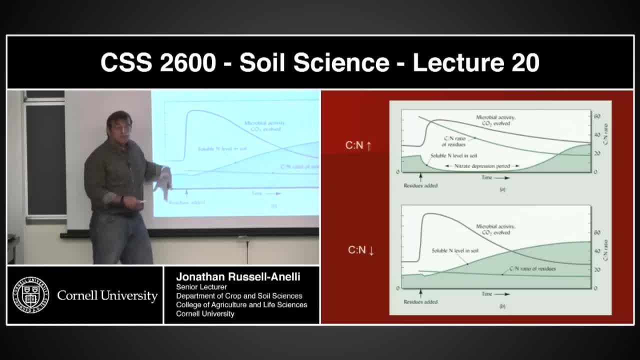 Okay, But you can notice, because the CN ratio is so low, the nitrogen is basically waste material in the carbon in that food that they're eating. They don't need that much. but remember this. Okay, My CN ratio is too low. I have to be blowing off CO2,, I have to be making ATP, all these. 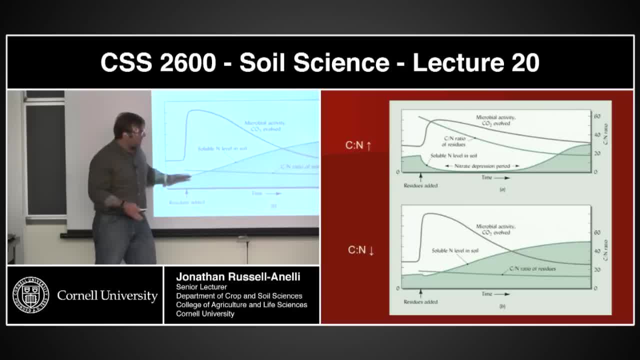 other things. Okay, I have waste material And that waste material is represented in the increase of the nitrogen. It's just available. Now that's available to all the other organisms, the plants that are in that system. Does that make sense to everybody? 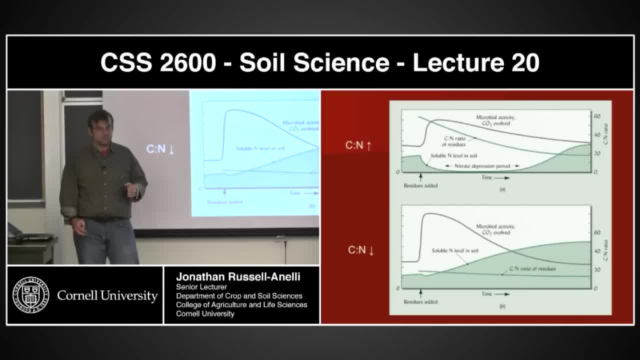 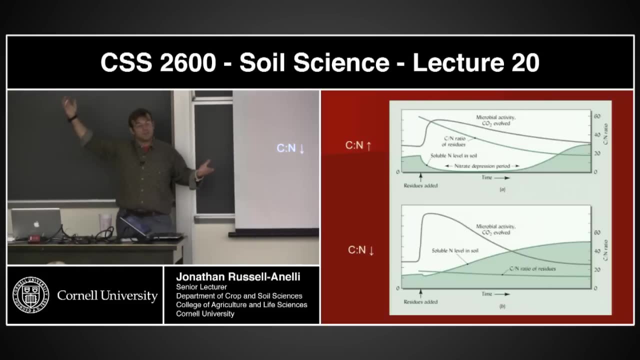 No, Yes Questions. Cool. Where's the original source of nitrogen? The original source of nitrogen would have been some place back here, some other organic matter that got added to the system. Now it also could be nitrogen fixation, but it's nitrogen that was added previously through. 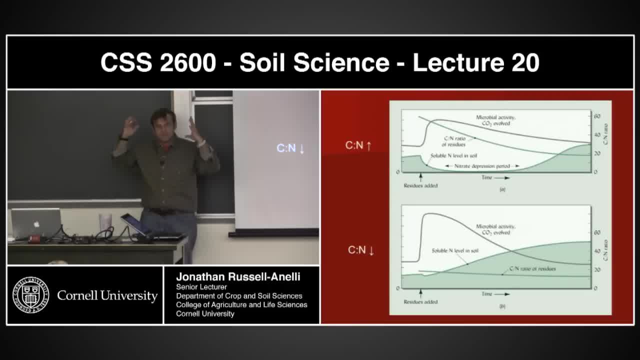 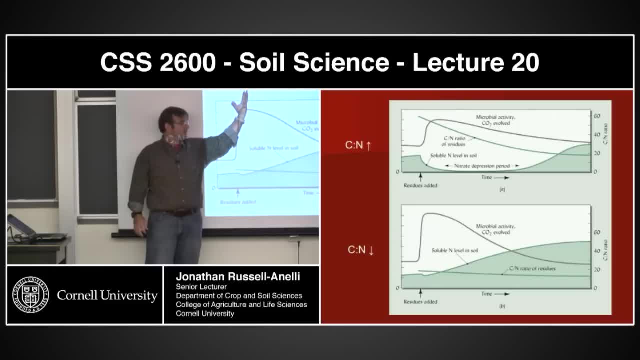 organic matter amendments: Okay. So imagine I had a leaf fall back here, Okay. And then we're basically looking this at the next fall, Okay, And the next fall I've got leaves, I've got leaves going in. The leaves have a fairly low CN ratio compared to wood. 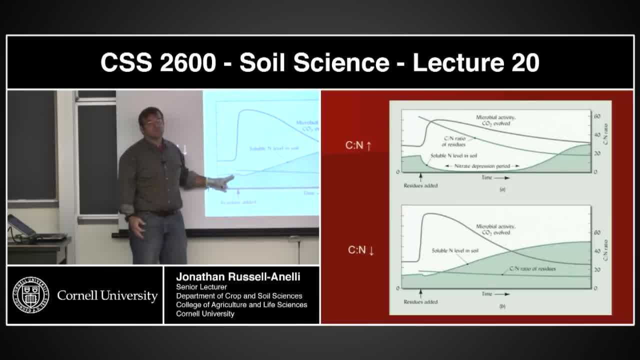 Okay, This was a tree fall, This was a leaf fall. Okay, So this pool is starting at basically the same spot because of the history of the site. Does that make sense, Lucas? Yeah, Okay, Go. So the nitrate depression period is that the nitrates in the rest of the soil like 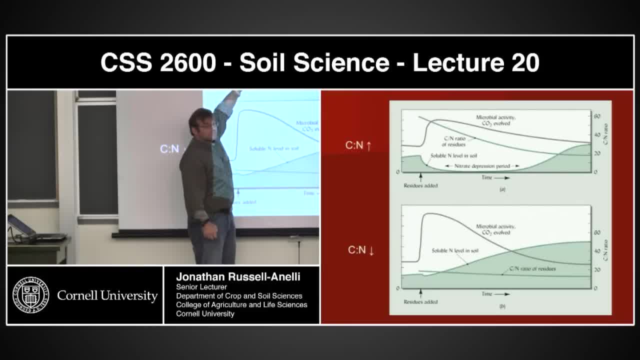 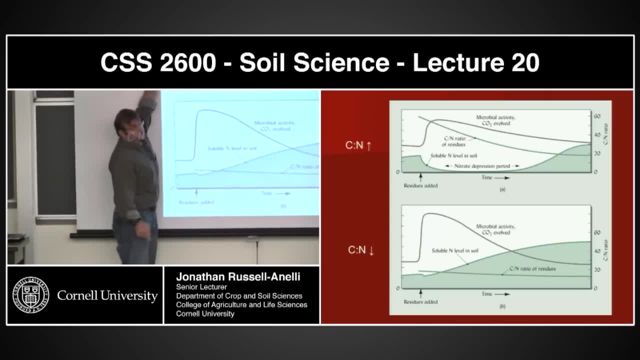 the microbes are actually feeding off of it and they don't have enough. That's the nitrate. Okay, So this nitrate depression period, So that's this nitrate that came in prior to the food. This is with the soil, Okay. 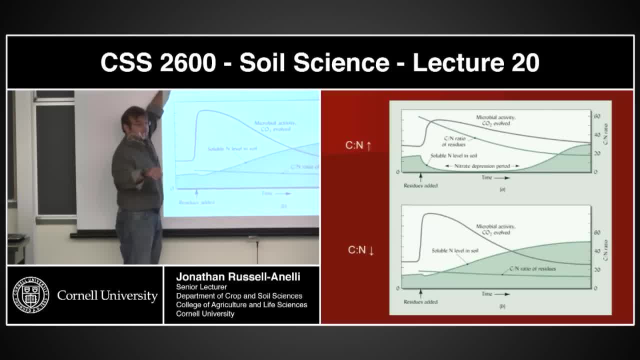 This is here already. This is not coming with the food stock. Okay, The food stock hits the ground, The organisms are going to start eating it. It's energy, But they don't have enough nutrients in that food stock and so they're going to harvest. 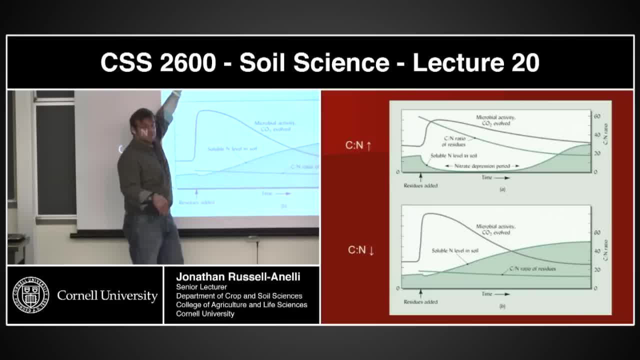 other locations, which is going to be the nitrate that's in the soil. Okay, So is that what you were talking about when you said like a nitrogen deficiency? This would be a good example of a nitrogen deficiency- The microbes. so this is exactly, this is the example of nitrogen deficiency. 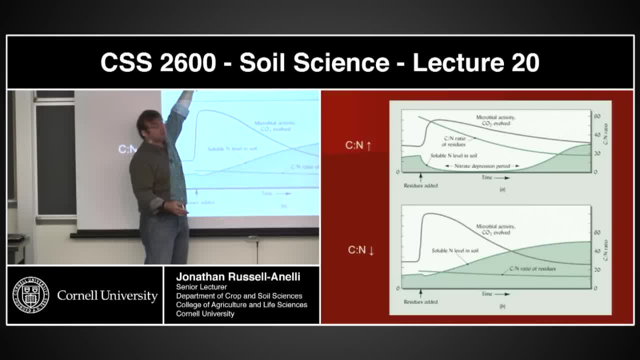 If this nitrate pool is depressed because the microbes are getting it and they are much better at getting it than everybody else- everybody else is now going to have deficiency in nitrate. Does that make sense? Now, somewhere down the line, those organisms are just going to start dying off, and once they start dying off, the CN ratios of the material that's being decomposed is going to start rising- or lowering, I should say- and as a result, nitrogen is going to be put into the soil, which then everybody else can get. Now it should be noted that this is a very localized event. 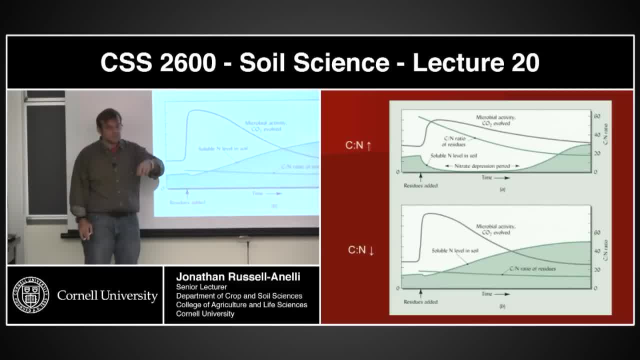 Where that food is is where the decomposition is going to occur. It's not like they're going to go out to the cookie mart to get nitrogen. Okay, They're going to. if the food is here, they're going to be depressed, the nitrogen is going. 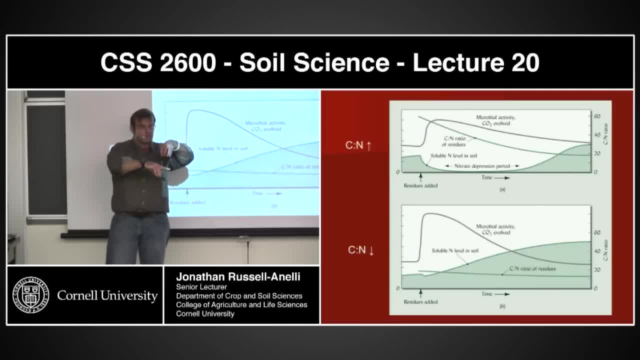 to be being depressed in this zone. Okay, If the material is a high CN ratio material. If, on the other hand, the CN ratio of the material is actually fairly low, this is where the nitrogen is going to be released. It's going to be fairly localized. 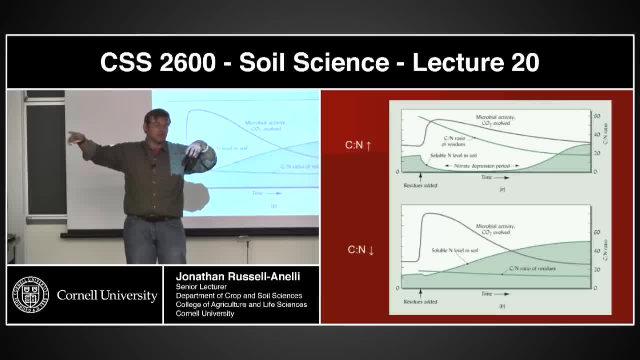 Okay, So the nitrogen isn't going to start well, it does actually migrate, but the nitrogen is not necessarily going to get over to the plant over there. It's going to be the plant that's over here that benefits from it. ie, when you put in: 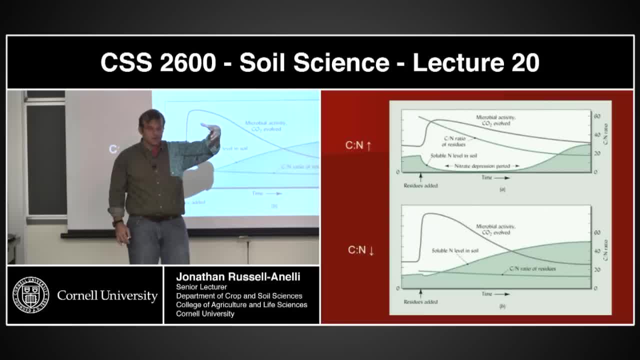 organic matter as fertilizer. you put your organic matter near where the organisms are that you want to take advantage of it. I don't put my compost over here and plant my corn over there and expect to get any response from it. Does that make sense? 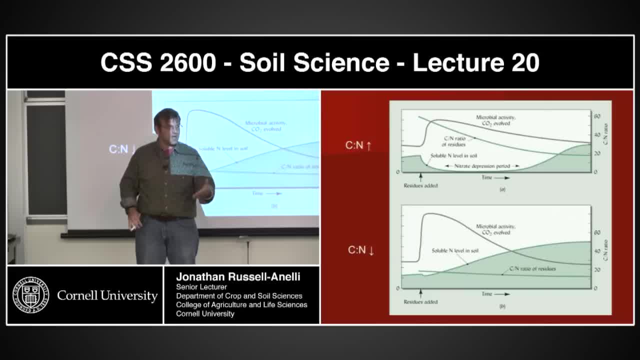 And that is actually a very good example of why location matters When you start talking about decomposition question: how does this work with nitrogen fixing organisms? So this is- this is actually a really good example. in this type of environment, Nitrogen fixing organisms don't have an advantage. nitrogen fixation- 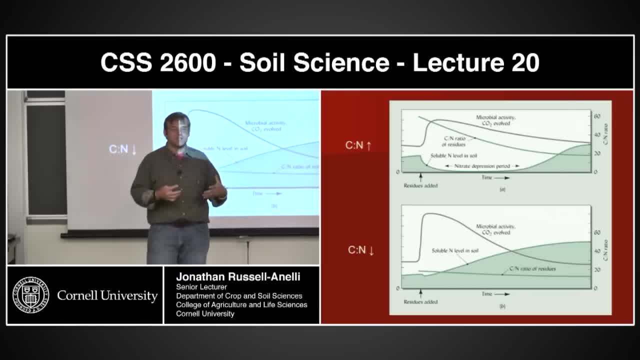 So the question is: how does this? how does this relate to nitrogen fixation microbes? There are a lot of organisms out there that have the ability To fix nitrogen. they take it from its mineral form and they immobilize it. They put it into a form that organisms can use, and we'll talk about this later in semester. 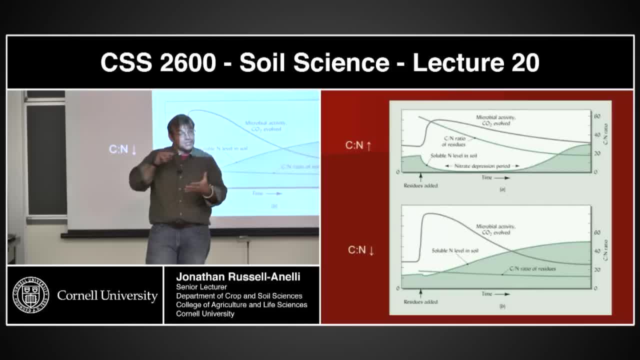 as well. But if the but to do that it takes ATP, it takes energy. So if there is nitrogen that's readily available in the environment, this is no benefit to them whatsoever. Why should they waste energy if nitrogen is already there? 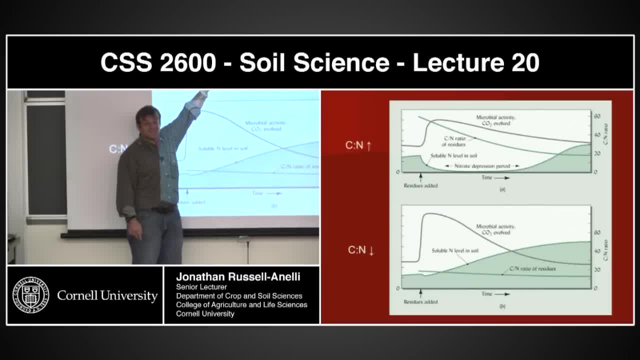 Make sense. On the other hand, in a scenario like this, where nitrogen is in competition, they can basically take nitrogen gas from the atmosphere and fix it into a biologically usable form. That's a severe advantage, a significant, not a severe. well, it is severe, a severe. 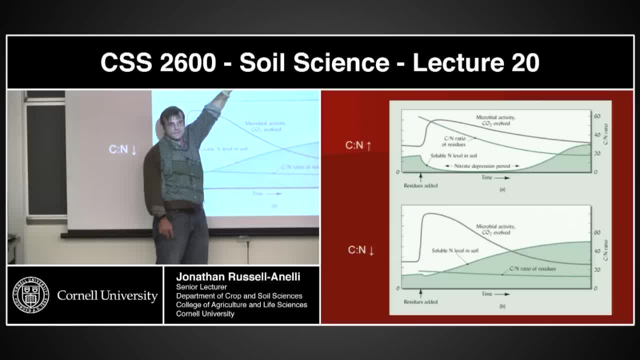 advantage in this type of environment because there are a lot of organisms that don't can't fix nitrogen And if you are an organism that can fix it, can take it out of the atmosphere and put it into a biomass form. you have a severe advantage. 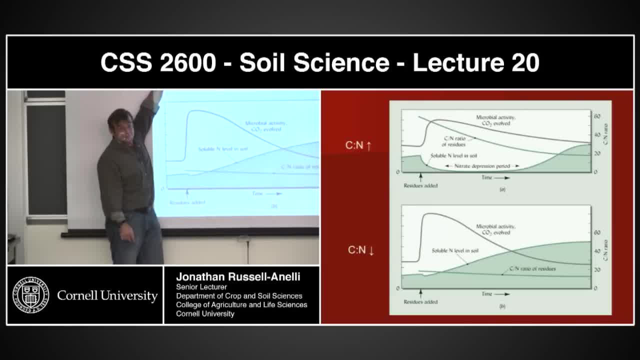 These guys, most of these guys, are taking. the nitrogen that's in here is already in an organic form. It's in a form that organisms can use, But if I get rid of that, there's nothing there for them to use. So in that case, those organisms that have the ability to take N2 out of the atmosphere. 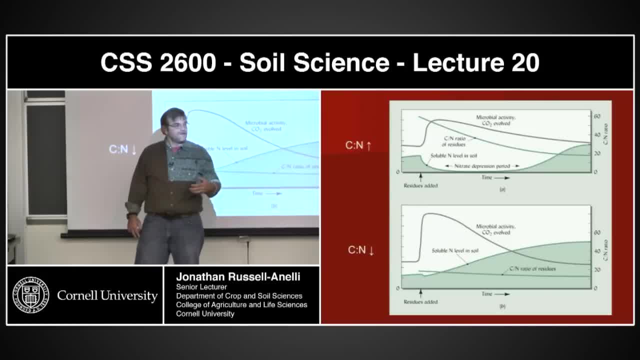 and turn it into an ammonium form, an amine form. That's a huge advantage. Now does we really? are going to be talking about nitrogen later in the semester, but does everybody have an idea about what I mean when I say they're fixing nitrogen? 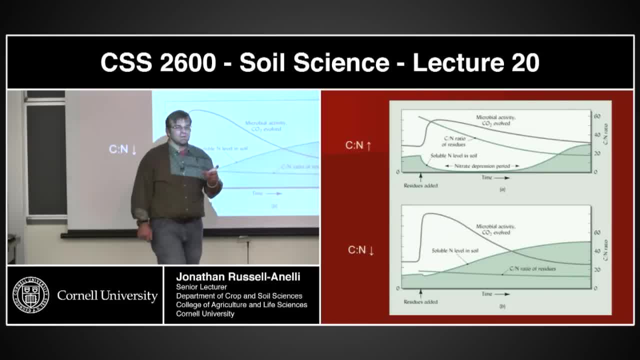 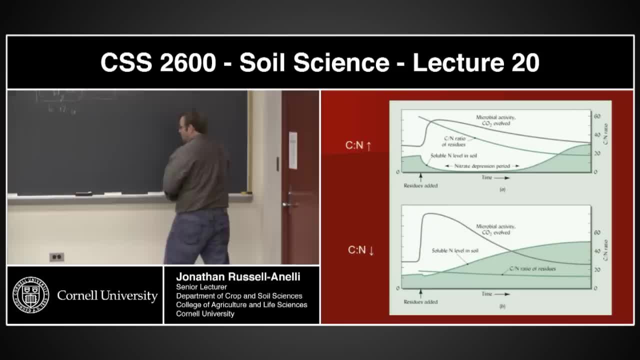 Sort of ish. I'm uncomfortable with the nodding that I'm getting here, So let me show you just we'll do this real quick and we'll talk about it later, a lot later in the semester- The nitrogen cycle. 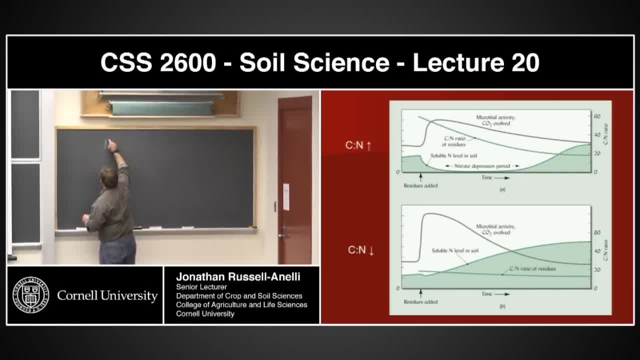 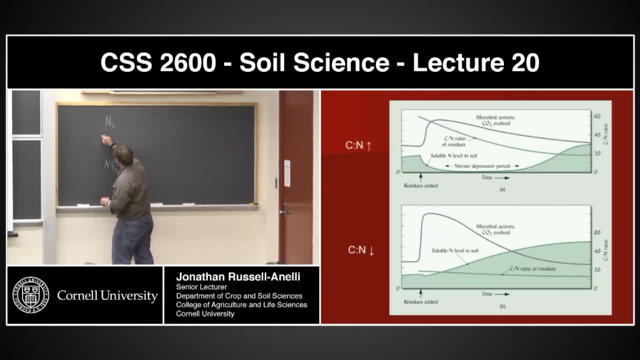 We're not going to talk about that. We're going to talk about it right now, But there's basically, for lack of a better, there's basically two forms of nitrogen that organisms can use and they'll convert it into amines and they'll basically- the amine is 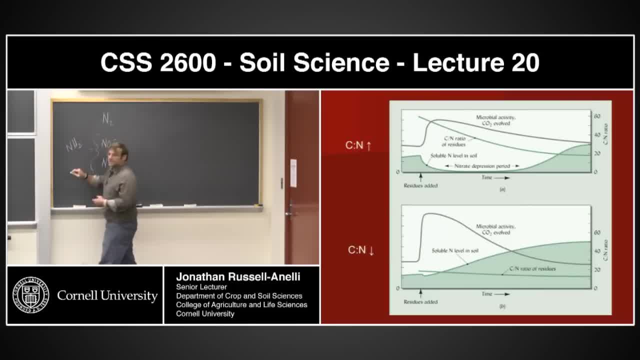 basically a form that's like this And that's: it's attached to a carbon structure part of the body. But they're doing it. they're basically taking these two forms. Now, not all organisms have the ability to take each one of these forms. 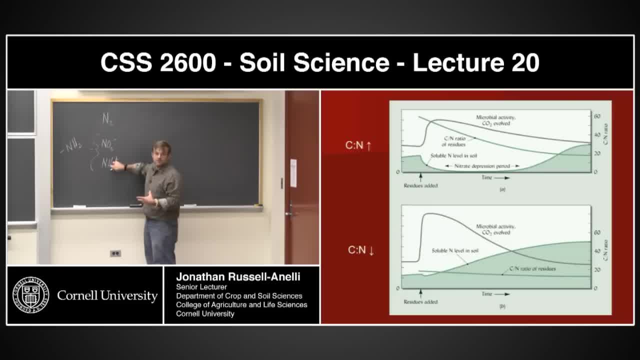 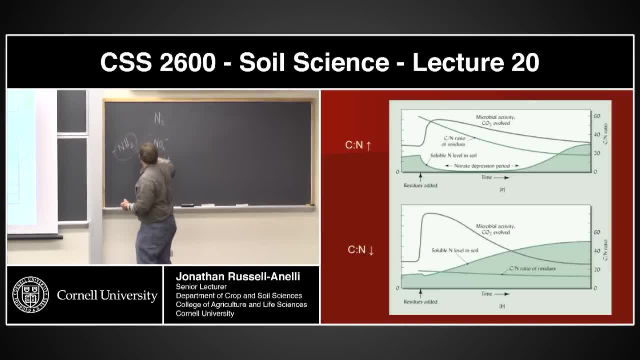 But plants do have the ability to take either one of these forms. Okay, This is the nitrogen that's being released through decomposition and it's coming out in these forms which plants can then take up, But there is an abundance of this in the atmosphere. 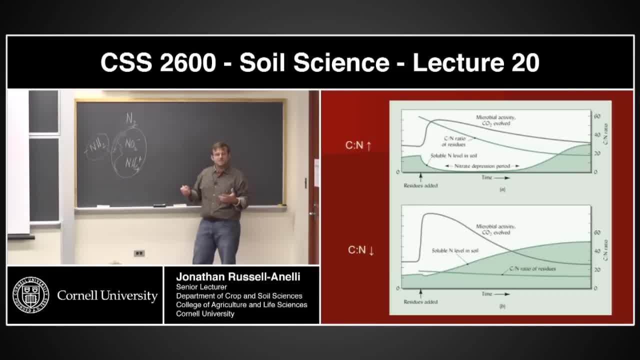 What is it Night? What? 80%, 79%, What is whatever? There's this huge number of nitrogen in the atmosphere, except it's in a unavailable form. The plants can't take it up- Why not? But there are organisms that can basically convert this nitrogen into these forms. for 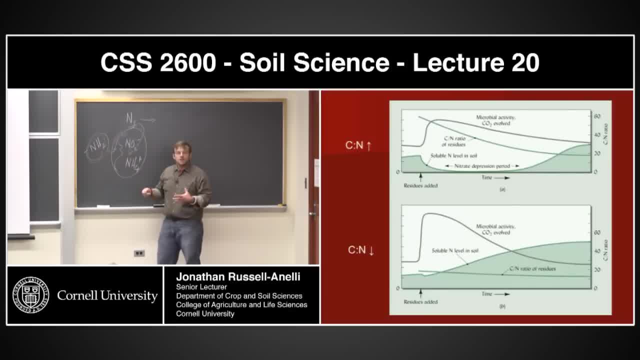 use. Actually they convert it into this form for use. Now they're in symbiotic. most of them are in symbiotic relationships with plants, where the plants are giving them carbon or energy and the microorganisms that are doing the fixing are giving the plants the nitrogen. 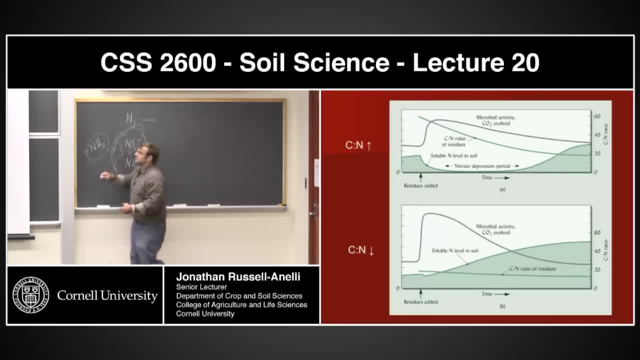 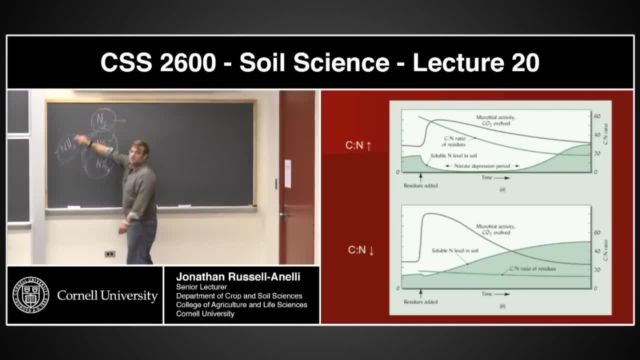 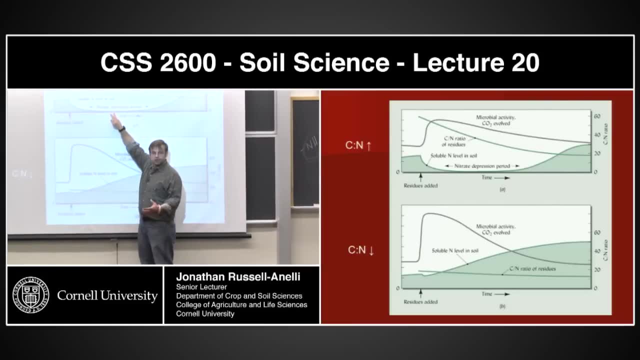 Okay, But if this is the nitrogen, that they is not available here? There is an abundance of this nitrogen and two gas in this environment, even when the nitrate is depressed. So, as a result, the organisms that can do that, they'll do this and they'll survive. 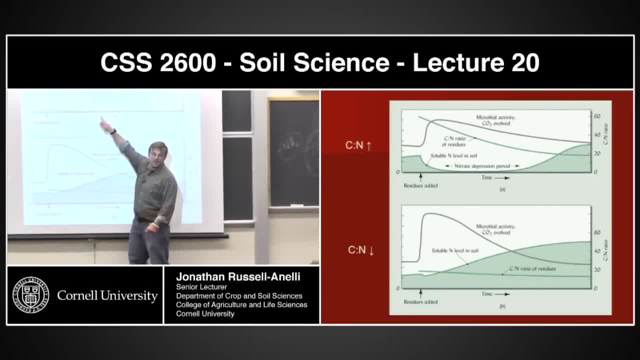 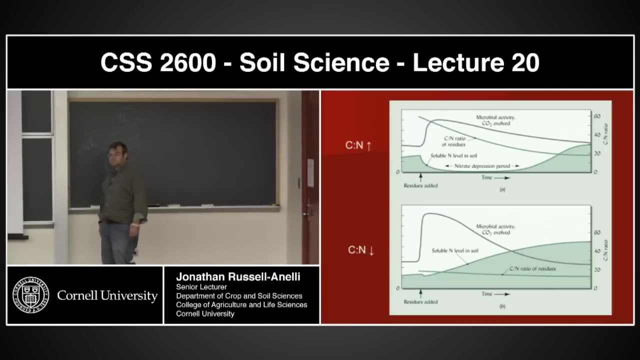 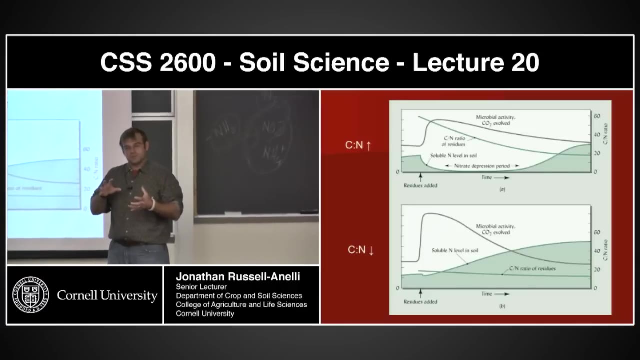 The organisms that can't do that and aren't as good as the microbes at getting this. they're basically going to go into senescence and potentially die. Does that make sense? Questions Go. I don't know if it's that they prefer it, but the relationship for nitrogen fixation. 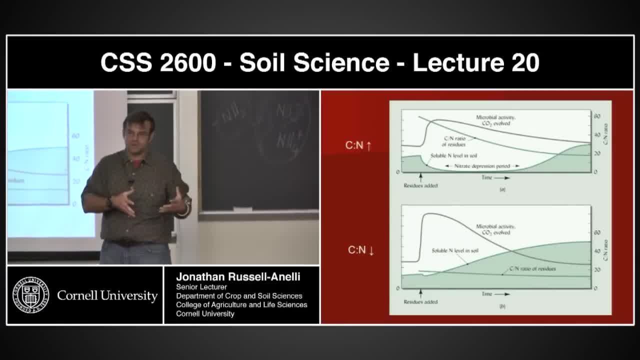 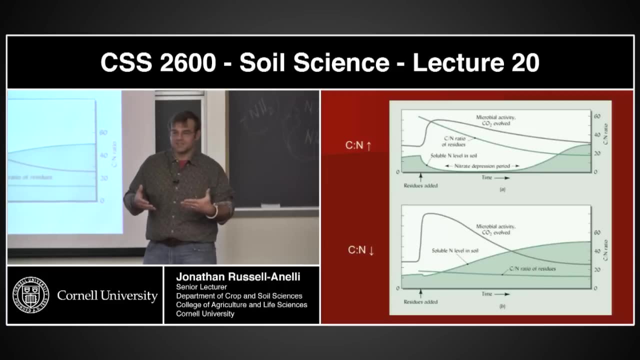 has developed in the legumes, while it hasn't developed in the corn. The symbiotic relationship between the microbial population and the corn has never been developed. On the other hand, I mean got a good analogy here, Good analogy. Can't think of a good analogy for this. 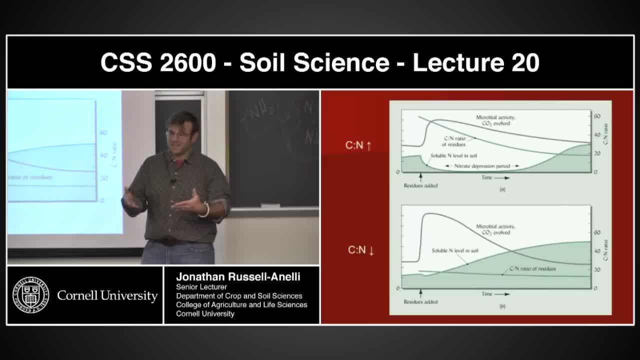 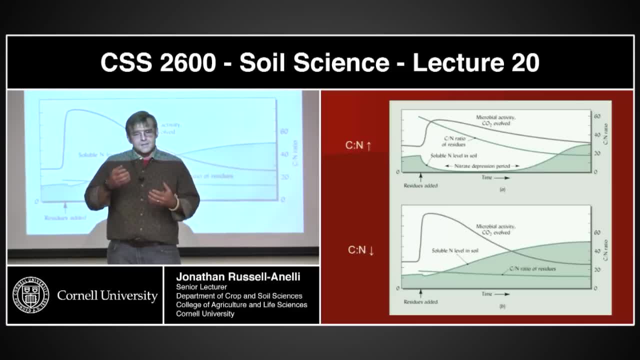 It's like pizza and beer goes really well together. Beer and cake doesn't go that well together. That's a really terrible one. The microbial population that has the ability to fix nitrogen. Some of them live in by themselves, but they- some of these guys- have redeveloped relationships. 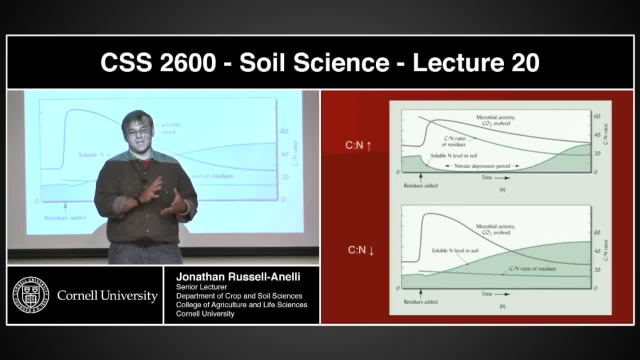 with certain plants, and corn happens not to be one of those plants. Okay, Whole slew of different types of plants. It's not just legumes, There's some trees and some other organisms, and there's also some fungi type of relationships as well, but corn just happens not to be one of them. 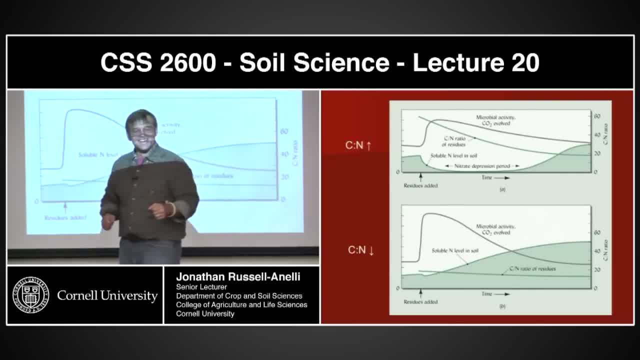 Good case for GMOs. You're going to go there. We were just talking about GMOs earlier- but this is not. we're not going to go that direction. Okay, Any questions? Does that make sense to you, Kind of. 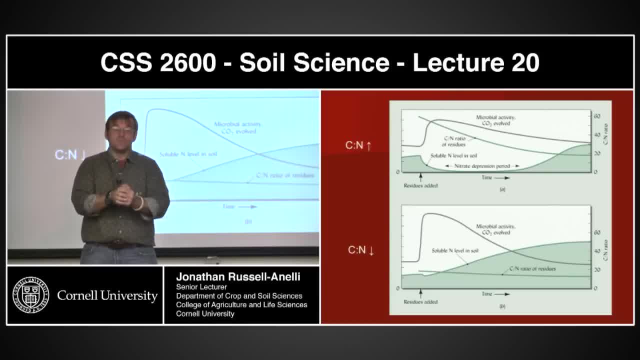 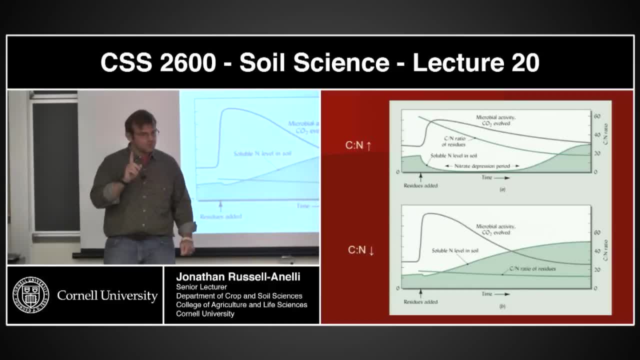 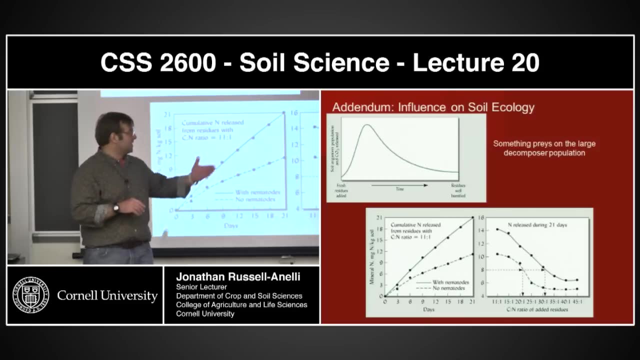 Yeah, Yeah, The beer and pizza one. That makes sense, right? Okay, Any other questions. on this one, We're fairly good with this, All right. Now I want to make an addendum here, and I think I've already actually made this addendum. 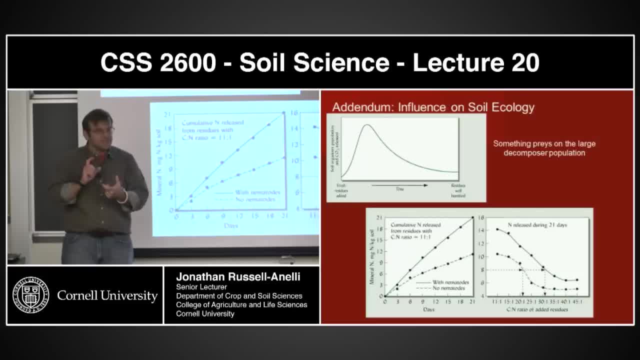 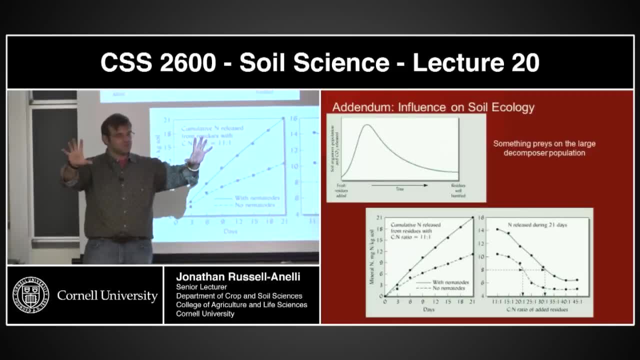 The reality is that this, this, is not living in isolation. Okay, The CN ratio is not. this is, I mean, we've portrayed it sort of as it's like by itself It's individual control. But the reality is that, if this is my population of organisms, 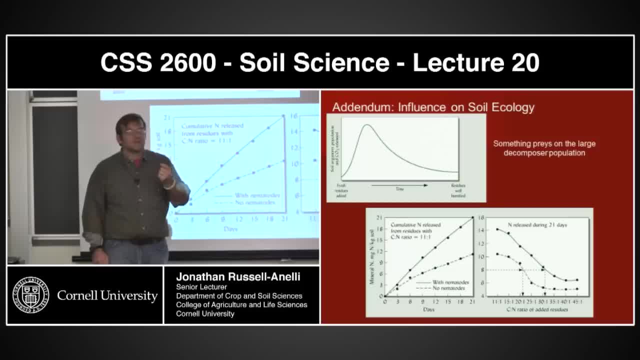 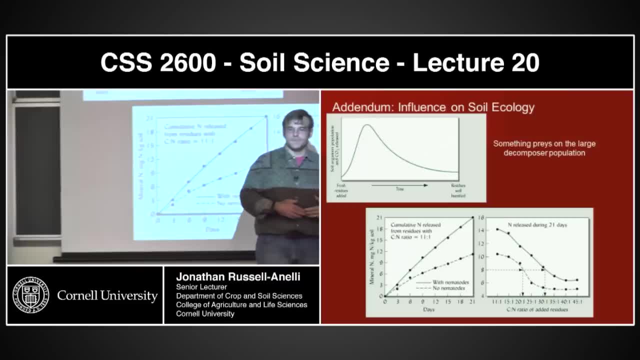 Here. this is a good one. I'm not sure I've got the right numbers, but if E coli, you guys know what E coli is: Microorganism, Very, it's a gut organism, but it's everywhere else. Okay If E coli were left to their own devices and nothing ate them and they never died because of their ability to replicate themselves to, I think within a week or something like that, That's an unbelievably small time. Within a week, the entire solar system would be occupied by E coli. 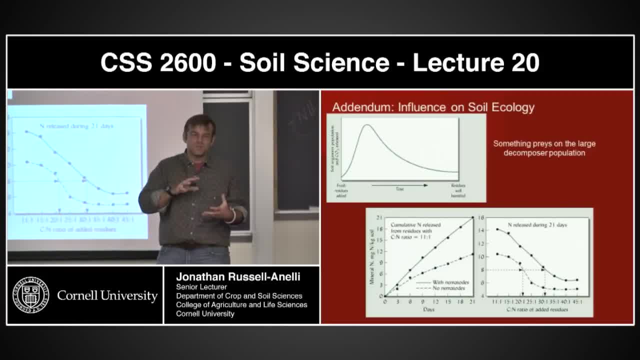 Something like that. It's some, maybe it's a month or something, but it's really this small number. So that gives you an idea about how the life span of these E coli, if they were immortal, Okay, But the reality is they're not immortal. 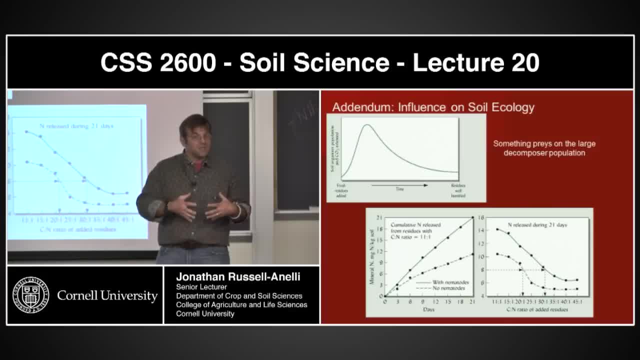 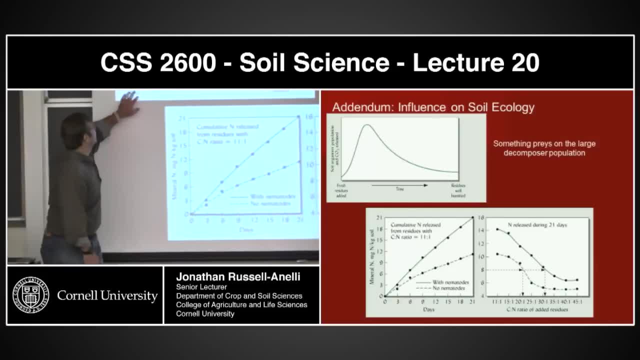 And then, most of the time, of course, they die of old age, but most of the time they're being eaten by something, because everything's a food for something, Right? Okay, So here's that fresh. you've seen this one before. 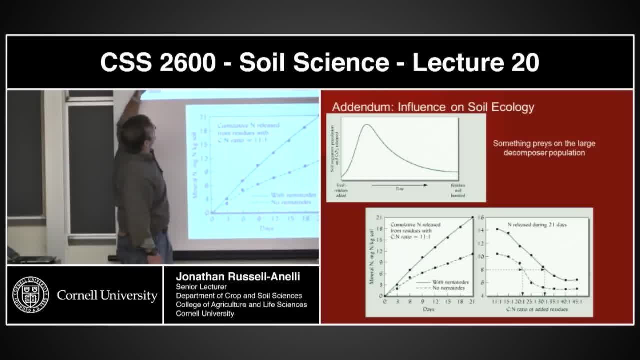 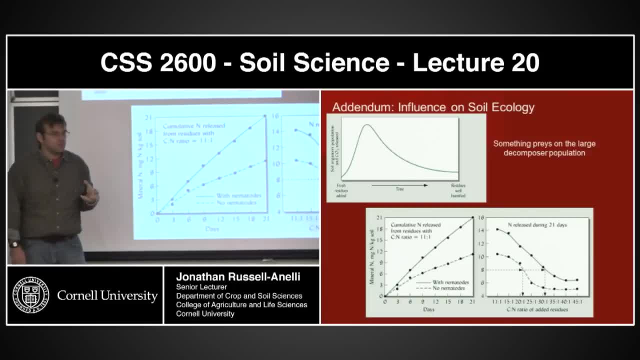 Okay, Here's that fresh material that's been added. This is the CO2 evolution basically, looking at the population. Okay, But that population drops Right. So what's happening in that population? Okay, That population is doing the decomposition of the CN material. 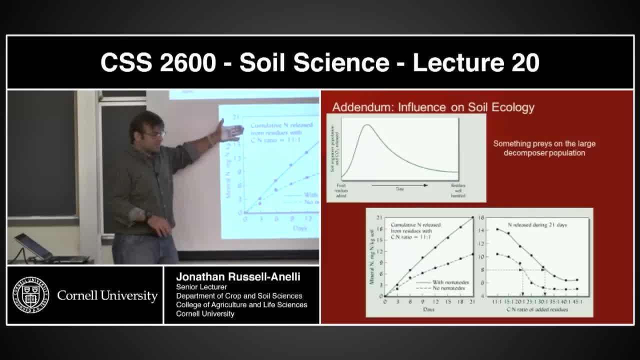 Right, Okay, But if we actually look at the amount of nitrogen that's being released from the soil, that's being decomposed or no, no, no, I add fresh material And I just have microbes in it. Okay, They're going to produce a certain amount of biomass and they're going to release a 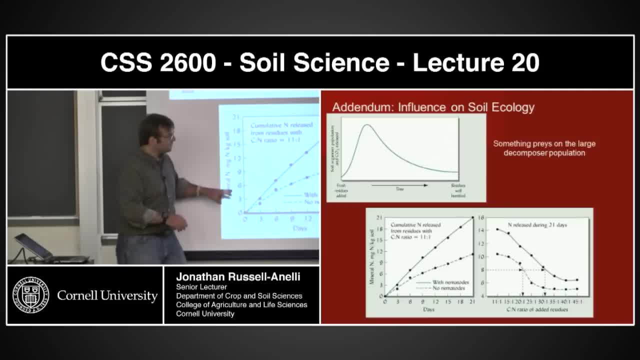 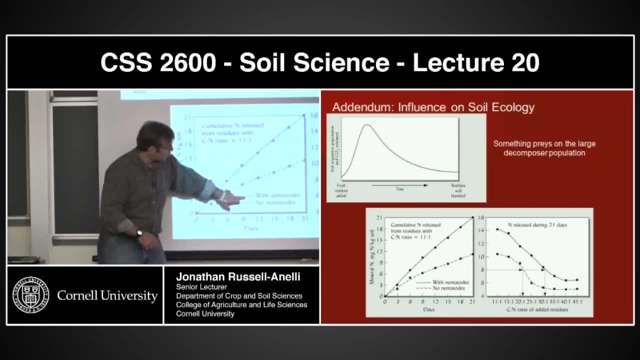 certain amount of nitrogen. They're going to mineralize a certain amount of nitrogen, Okay, And that's what these lines basically represent here. This is mineral nitrogen that's in the soil over periods of days. Okay, This dark line right here is with nematodes. 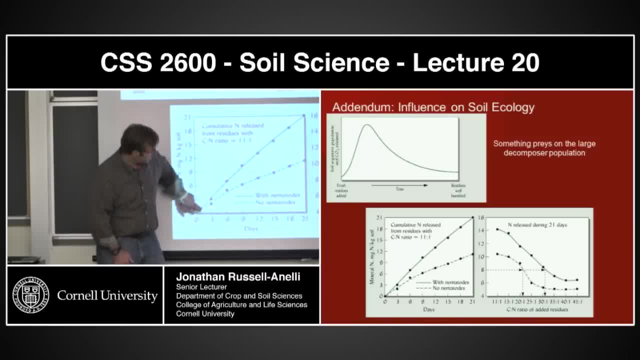 This dashed line right here is: with no nematodes, Okay, And you'll note that without the nematodes, there's a lot less. There's a lot less release of nitrogen into the soil system. Okay, So if I did not have nematodes, this is how much nitrogen would be released in the system. 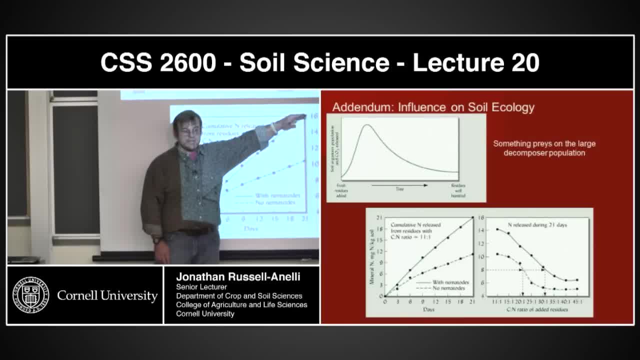 With nematodes. this is what's being released Now. nematodes are sort of predatory little worms type things And basically what they're doing is they're eating this population And in the process of doing the eating, they're breaking them up and they're sloppy eaters. 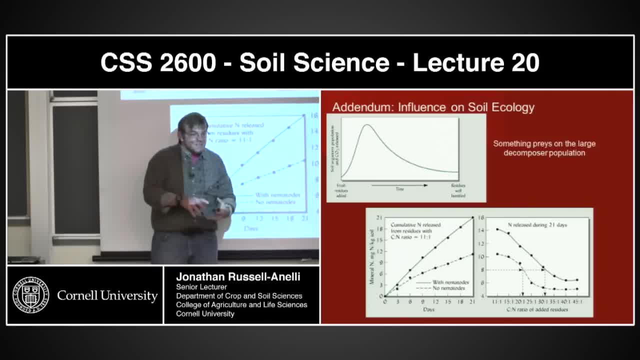 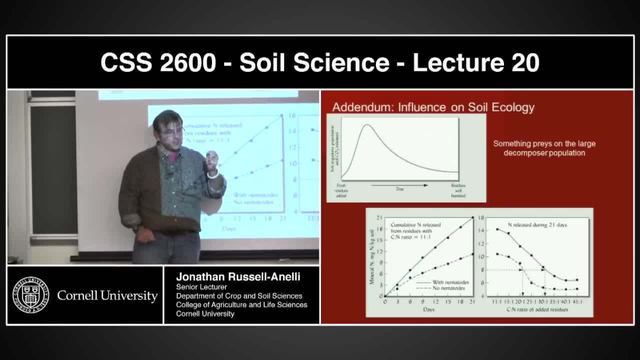 just like us, And that nitrogen that's in the biomass of the microbial population is being released. So it's not simply a relationship of the decomposers and their waste products. It also has to do with the whole trophic structure of the soil has a huge influence on how much. 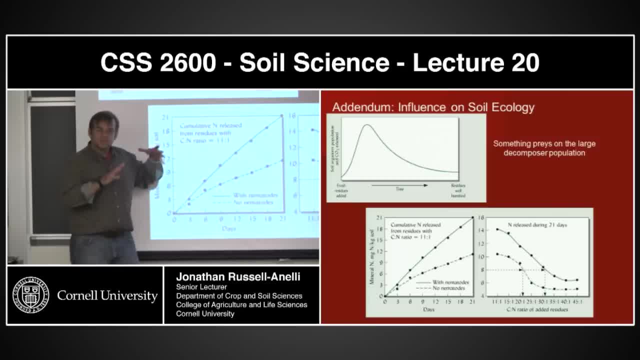 nitrogen is actually released, And the take home message of the slide is: don't just look at CN ratios, You also have to look at other things. Okay, Placement being one of them. Okay, Does that make sense? Okay, Questions so far. 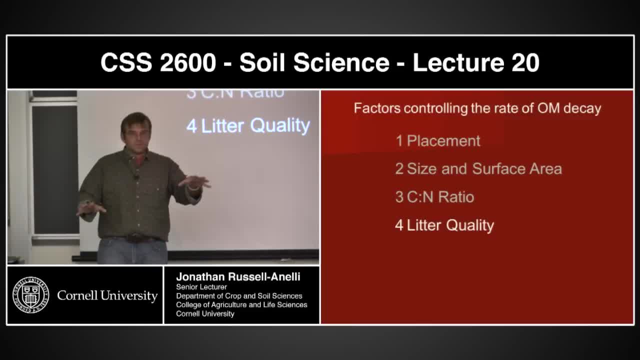 Cool, All right, We're going to take the last section and that's basically litter quality. And the truth is that CN is part of litter quality. Okay, But we pull it apart because it's an important feature by itself, Okay. So litter quality. 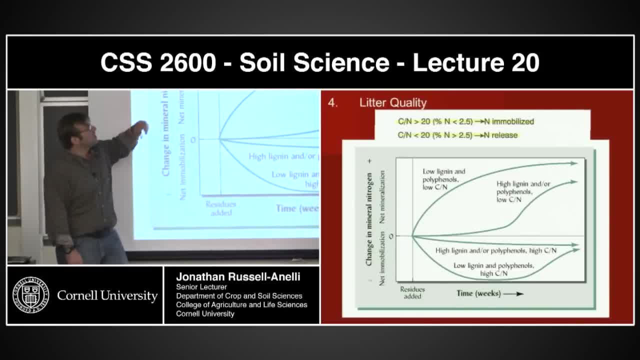 Okay, Here's those CN ratios up at the top: CN ratio greater than 20.. I'm having N mobilization CN ratios less than 20.. Okay, Less than 20,. I'm going to have nitrogen release mineralization. 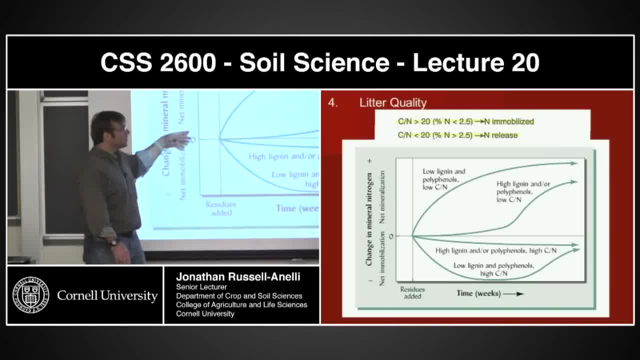 Right, Make sense, Okay. Well, let's take a look at CN ratios of a variety of materials. Okay, The rule of thumb is: high CN ratio is going to mean that I'm going to have N immobilization. Low CN ratio, I'm going to have N release. 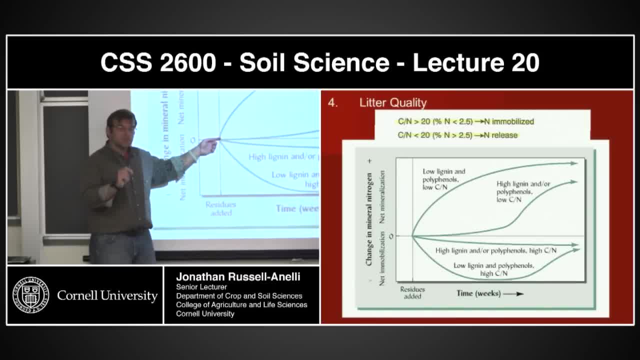 But just because I look at those numbers, I also need to look at the structure of the material that's being decomposed. Okay, So this stuff up here, these are low CN ratio stuff. This is high CN ratio. This is time on this track. 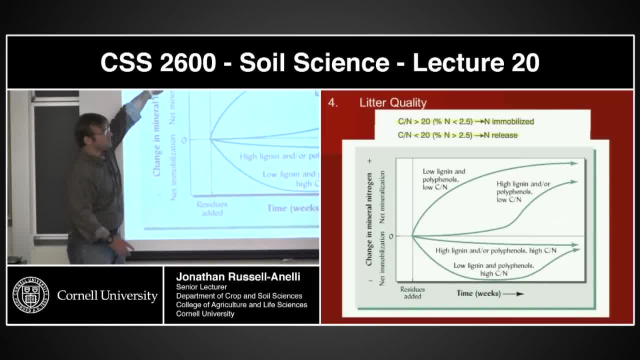 And zero here represents the point at which above I'm seeing mineralization, below I'm seeing immobilization Below. immobilization, meaning it's going into the biomass, It's being taken out of the system. Mineralization, meaning the nitrogen is being released into the system for everybody else. 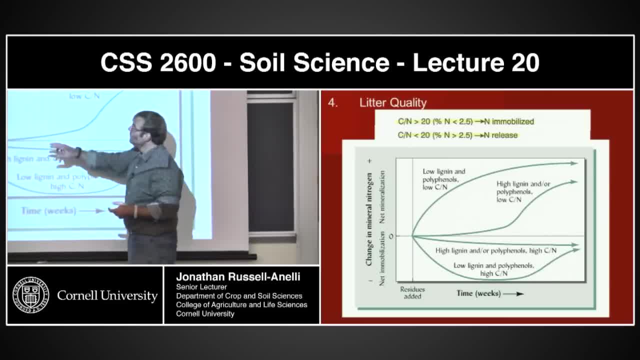 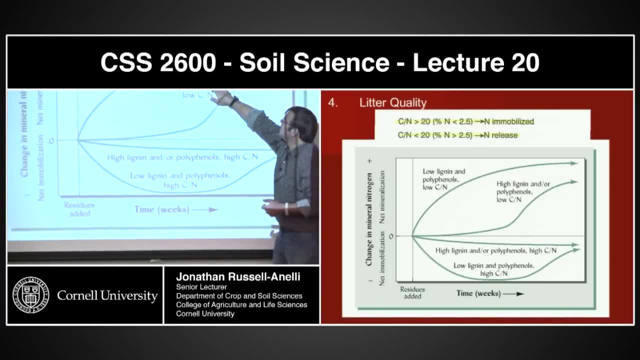 Okay, Now I have four different materials here. This is straight out of your book. I have a low lignin and phenolic materials low CN ratio. I have high lignin and or polyphenolic materials with a low CN ratio. I have high lignin and low lignin with a high CN ratio and a high CN ratio. 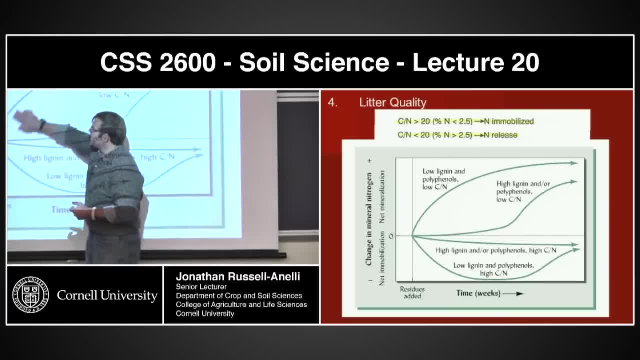 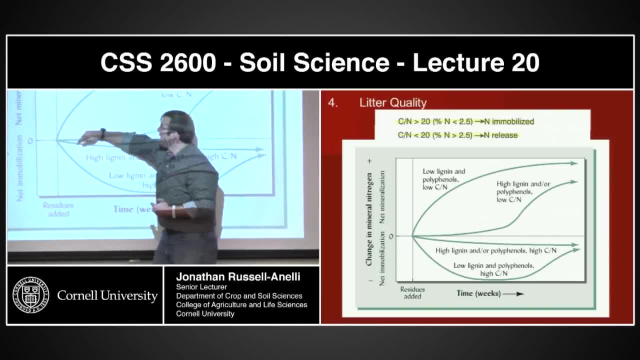 Okay, Look at these green lines and they basically: this is, this is time, So the quicker it moves up, the faster it happens. Okay, And the distance here is basically we're representing how much Mineralization or mobilization occurs. 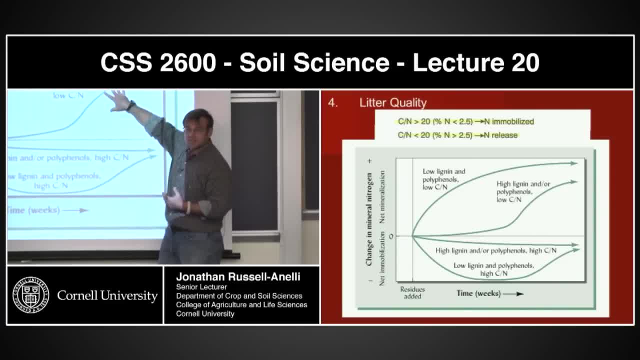 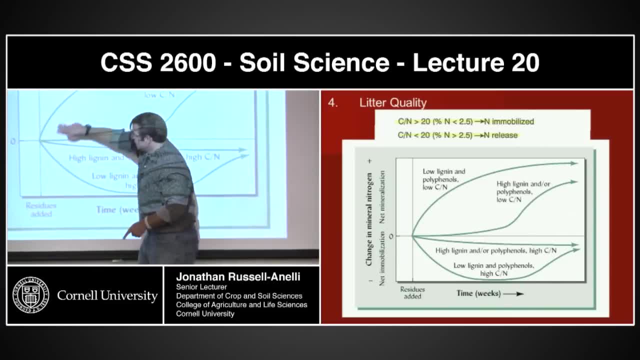 So just because you have a low CN ratio doesn't necessarily mean I mean, this is the class of these two lines here. What we would generally would think of: Okay, This is low lignins, This is low lignins as well. 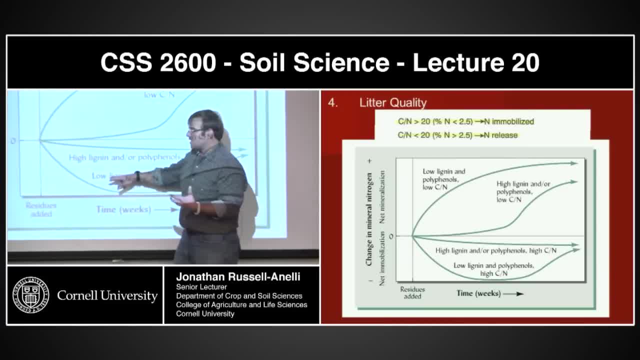 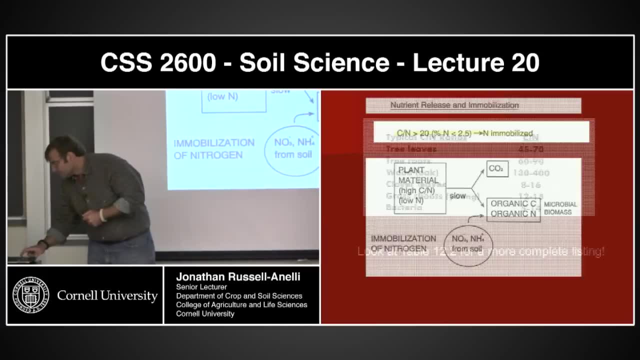 Lignin content. the ability of the material basically represents, or the structure of that material. Basically that represents how fast it in fact can be decayed. Okay, The the. I don't know if I still have this, Did I keep this? 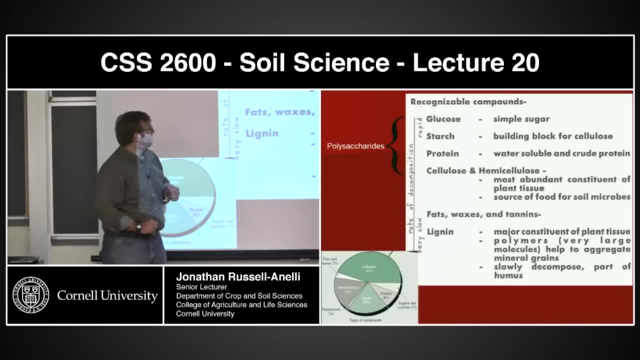 Remember this slide. So if we think about the material and how fast it decomposes, in general, this is not necessarily true. In general, we think of the glucoses being simple sugars- They're going to be easy to decompose- The lignins being very complex molecules, being very hard to decompose. 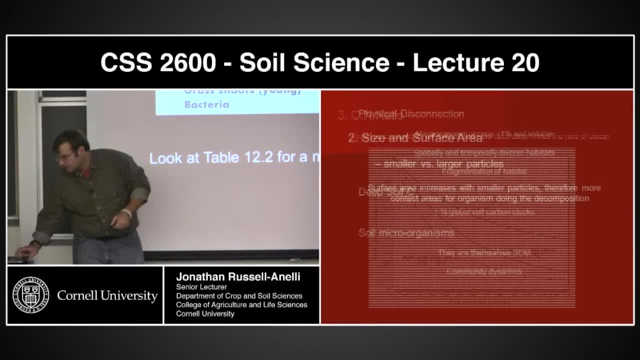 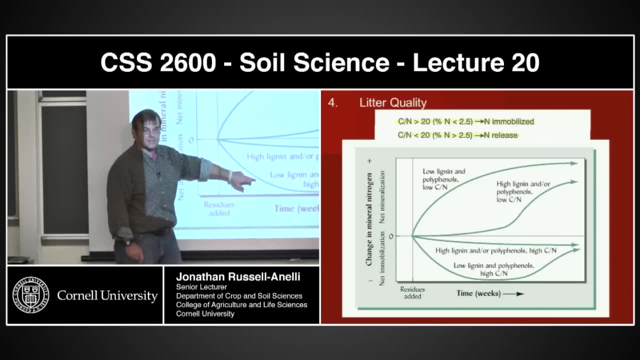 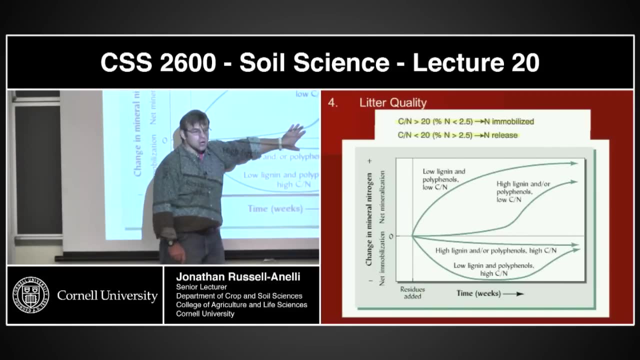 Okay, Now go back to this slide. Low lignin, low lignin on the outside fast to decompose. The inner two have high lignin contents and so, as a result, they take longer to decompose. Yes, they both have the same CN ratio as these guys and they, in general, end up at the same. 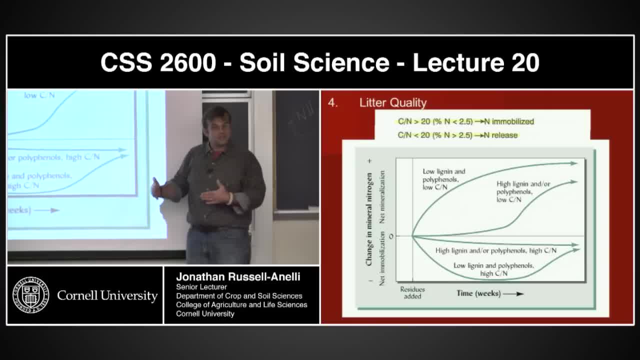 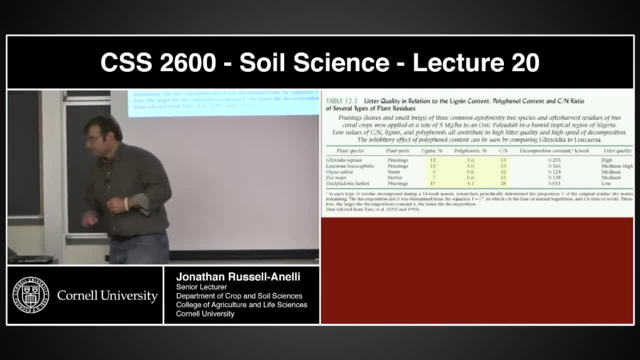 point, but it just takes a different time scale for them to get to that point. Does that make sense? Yeah, Now if we look at a lot of different materials, I don't know if, can you guys actually see this slide? 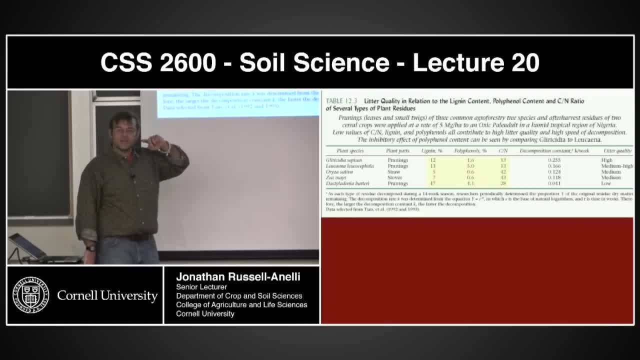 It's in the, in the PDF that you guys have. but basically, what you're looking at here is a variety of different plants, Okay, And it tells you what the plant parts are, but what it shows here is lignin versus polyphenol. 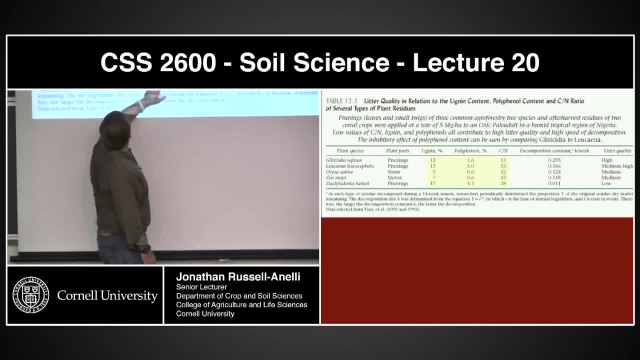 content, So higher numbers. this one has a really high number, has a high, fairly high number of polyphenol And basically it shows you the CN ratios. Okay, This is lignin. It's CN ratio is 28 to 1.. 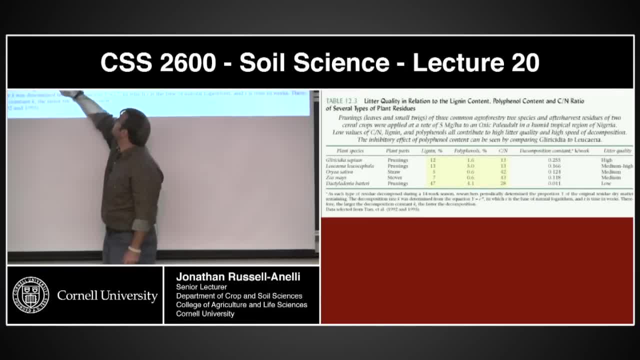 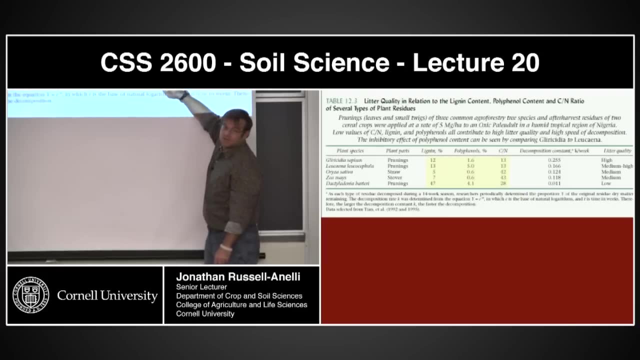 This has a very small amount of lignin, basically 7%. It has a ratio of 43 to 1.. Okay, Now, this is a con. this constant is a decomposition constant constant. Okay, The higher the number, the quicker it decomposes. 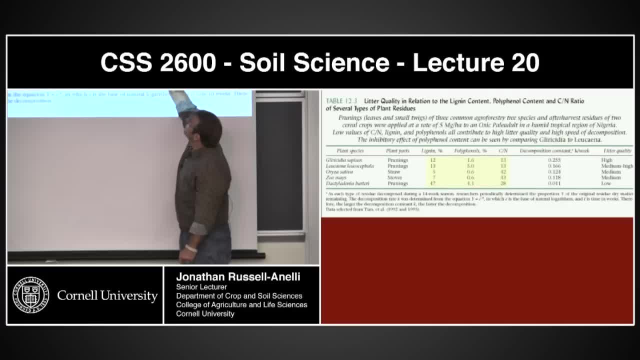 Okay. So looking here at this 13 to 1 material, it decomposes very quickly, but these 43 and 42 to 1s compared to the 28, these guys decompose a lot quicker than this. So it's not the CN ratio alone. 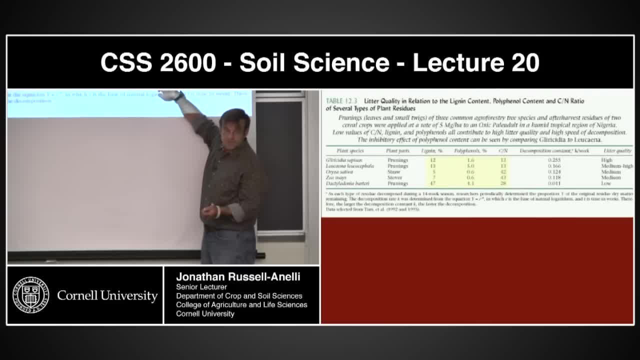 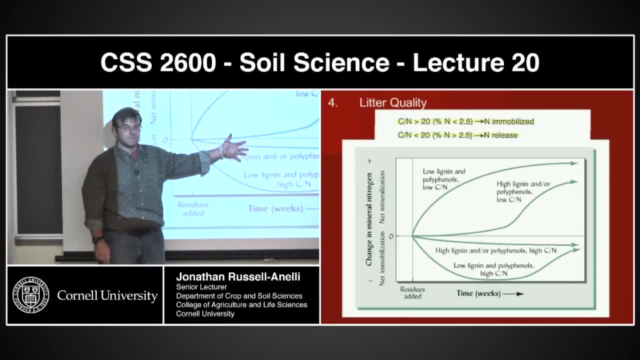 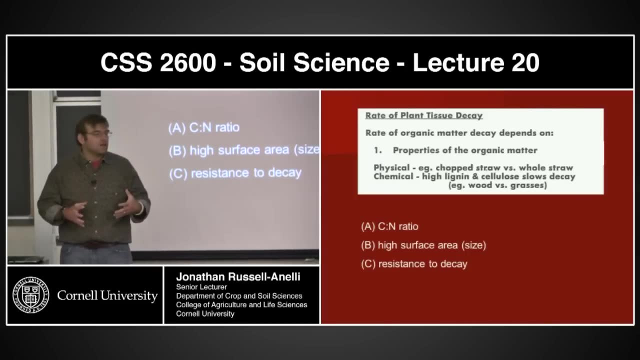 It's the structure of the material. Does that make sense? So, in essence, this is the data that filled in this chart. Okay, Now we've talked a lot about the placement you know: CN, ratios, size, litter, quality. 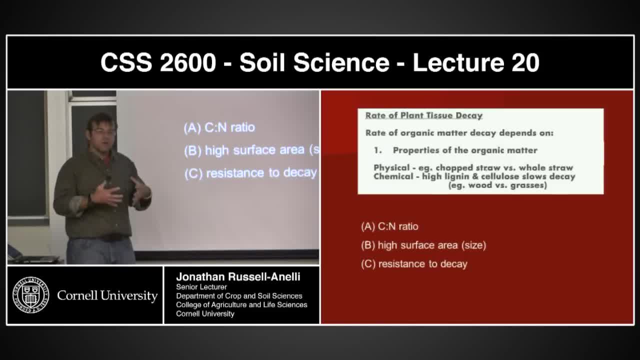 What is it if we're looking at decomposition? what is it that actually is? when you look at everything together, what is it that's controlling those rates? It really is the property of the organic material, where it happens to be the CN ratio of it. 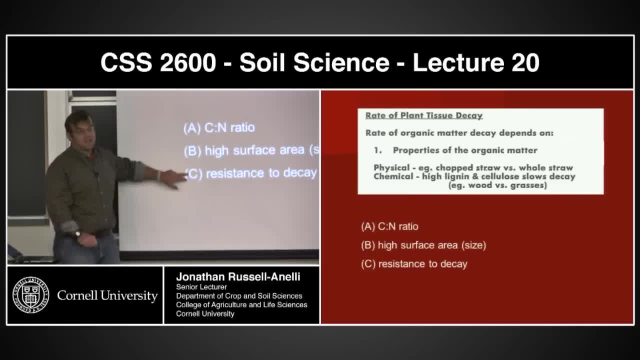 the surface area of it and its resistance to decay. Now, the truth is that, all of these combined, it really is where it is located. It's location, location, location. But it's this combination of different things that controls this decomposition.